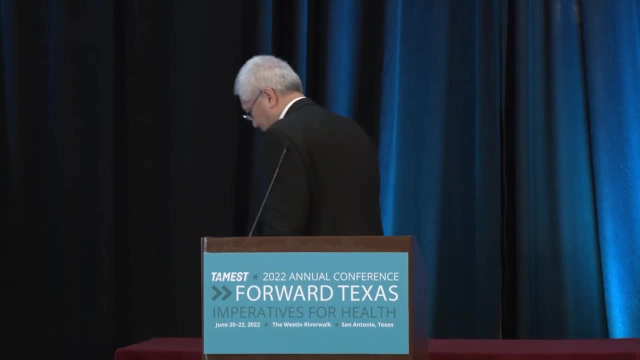 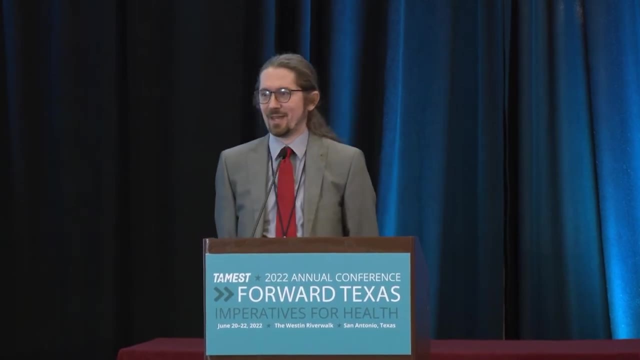 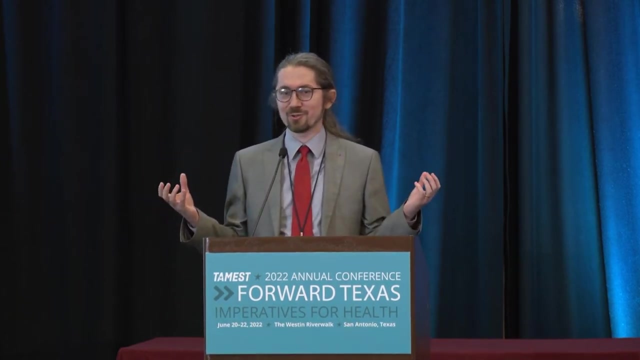 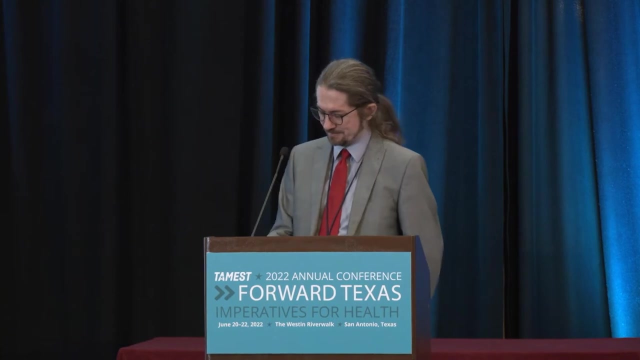 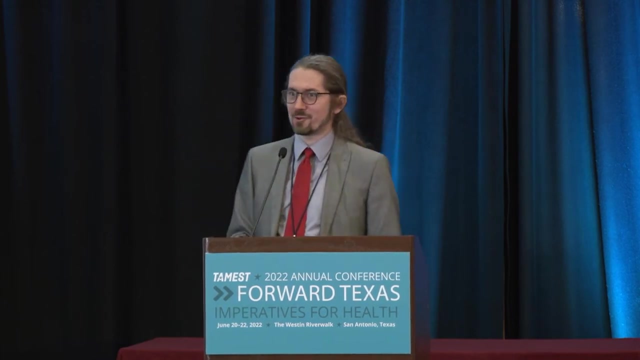 the University of Texas at Austin. Thank you so much And I'm delighted to be here and I'm extremely excited to inspire our thinking about indoor air quality today. So I would like to acknowledge my wonderful research group, graduate students and postdocs. 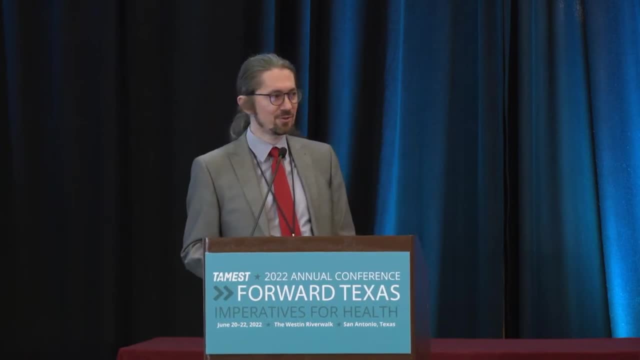 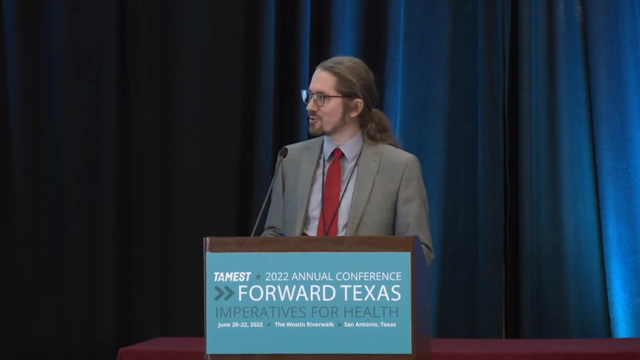 and also like to thank a lot of sponsors who have generously funded my research. And I will start from the question: Have you ever wondered how much time we spend indoors relative to outdoors? Well, it turns out that the total time spent indoors is approximately 90%. That's shocking. 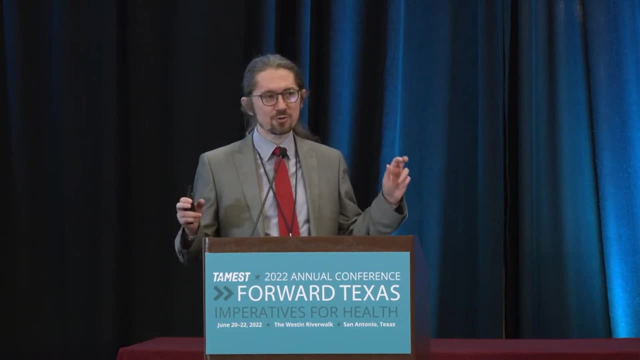 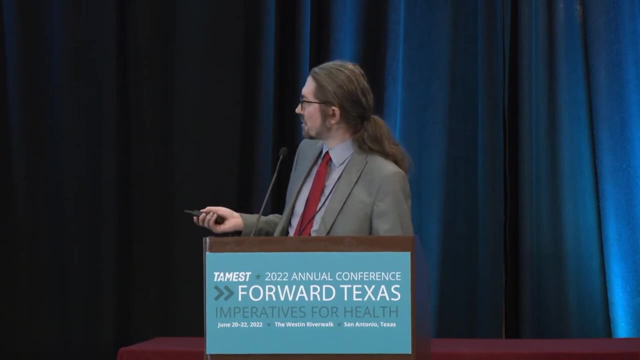 And it can be converted to so-called Corsi code. And this is what do these numbers mean? So these are years. So 79 is average life expectancy in the US, out of which we spent 69 years indoors, 54 at home, 26 in bed, 4.3 on a commute and actually, 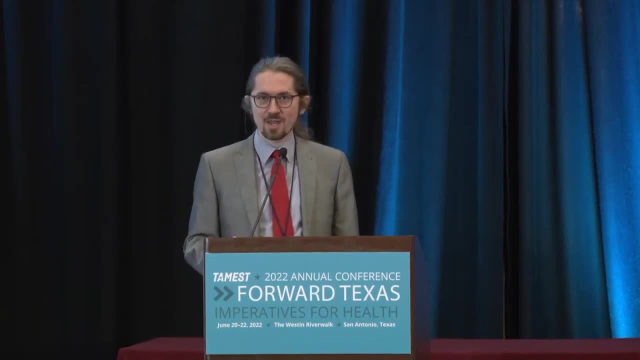 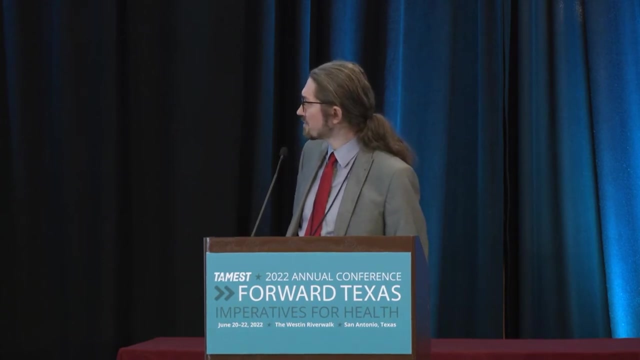 only six years in total for outdoor air And we worry about relatively clean outdoor air quality, which is regulated, and often not worry so much about indoor air quality, which is unregulated. So indoor well air quality is among three out of 30 causes of global ill health. 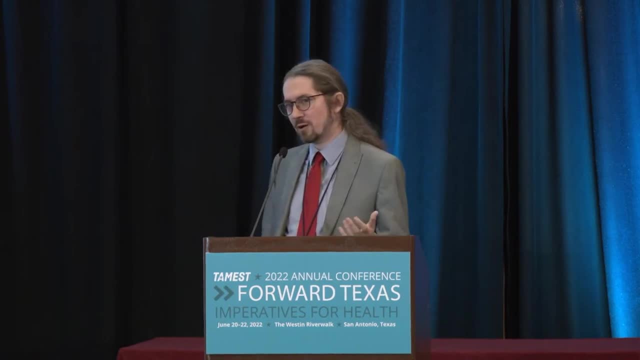 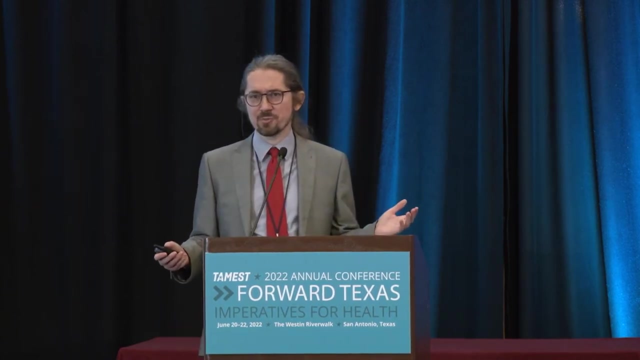 It's about 10%, And what I want to highlight is that exposures to adverse air quality occurs predominantly indoors, And this is an interdisciplinary problem and it requires collaboration between engineers, chemists, physicians, clinicians and so on, And there is a lot of opportunities here to close the gap when 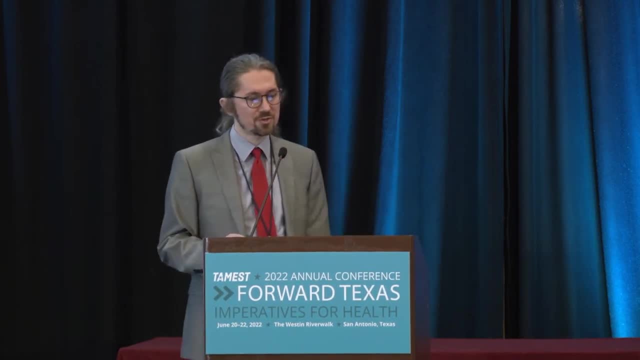 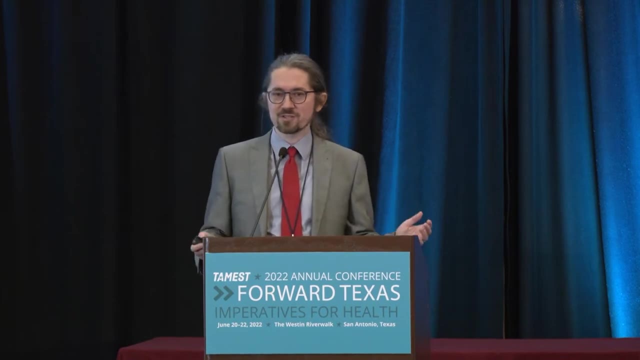 going between source emission rates to actual health effects, And one of the landmarks of public health research is the famous six cities Harvard cohort study, And this study showed beyond doubt the link between air quality and human health. So as you can see here, for example, the cities that 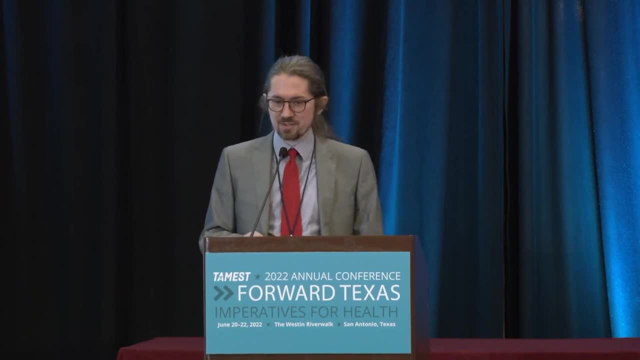 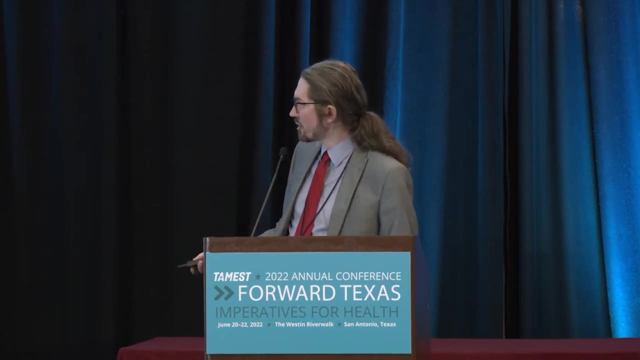 had most. they were most polluted. the survivability rate is much, much shorter. But did you realize that when you eat, when you prepare a stir-fried dinner, for example, the concentration of particles- and it's just fine- PM2.5 particles, which is a fraction of total particles, can be so much higher? 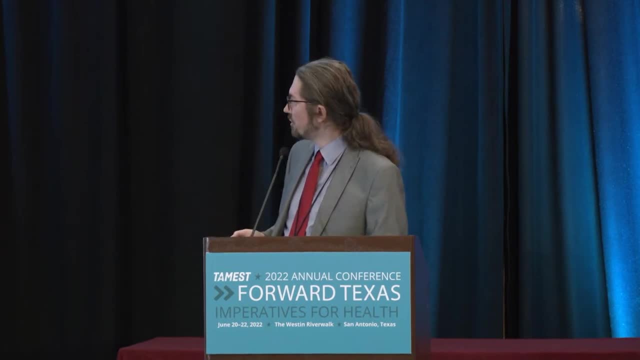 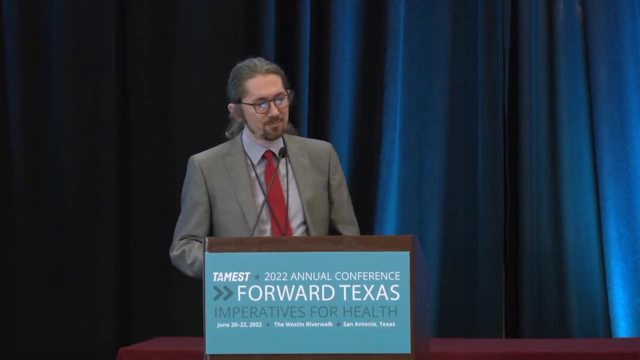 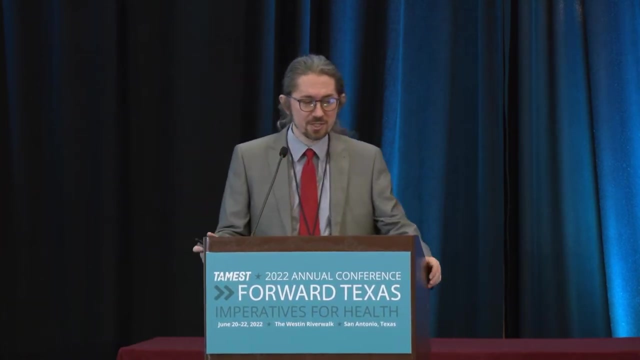 And I know it's acute, but this is what we don't think about. So I'll tell you a little bit more, And I will start from particle exposure. So we know that there is an impact on mortality, and the recent Lancet article mentions that. 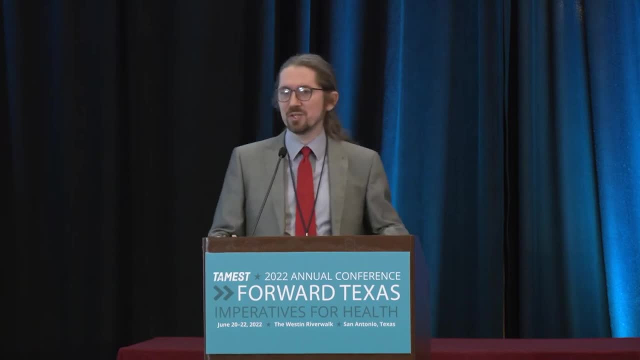 there are approximately 2.7 million deaths due to indoor air quality. So to understand the health effects, we need to understand how the polluted air gets inside the air And what happens when the air becomes colored through intake. destaulias are they, apparently? allowed to be constructed in other satellites. How can that happen? So after four years, we better investigate. So I can think at this time whether they should be detonated or not. either an earthquake or, if they're not, another life event or no. Much is impossible. but 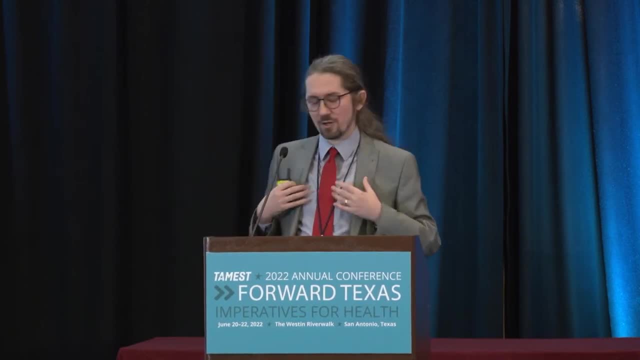 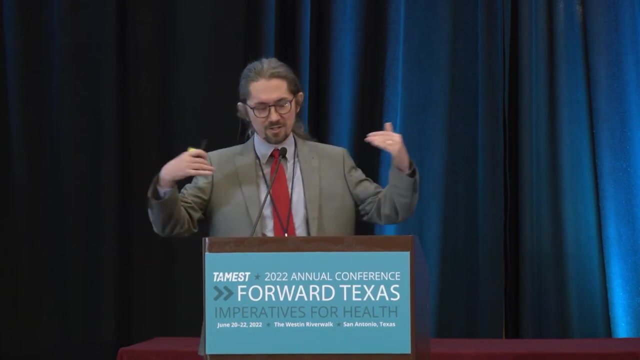 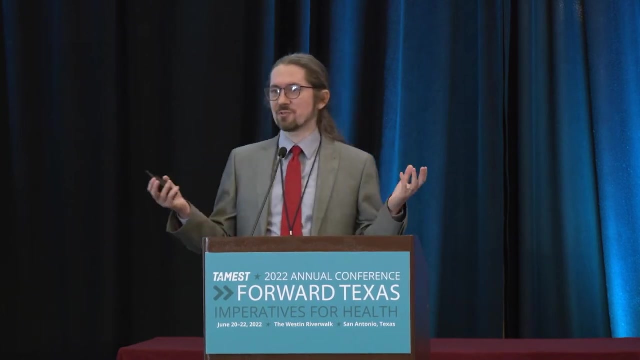 into our body through this nice system of our lungs. we have about half a billion alveoli in lungs where the gas exchange takes place, So with half a liter inhaled with each breath. we also inhale indoor pollutants, So there are thousands of different chemicals. 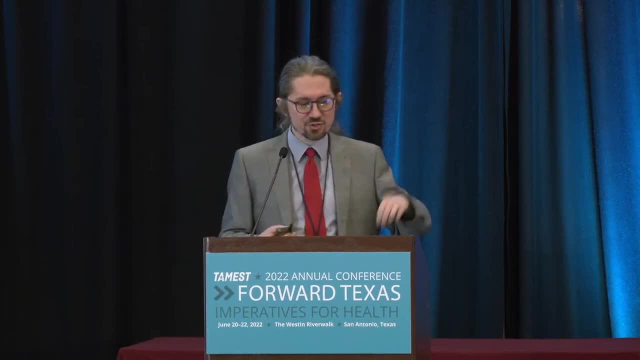 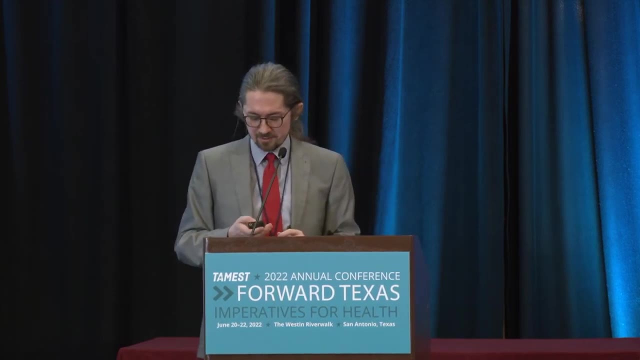 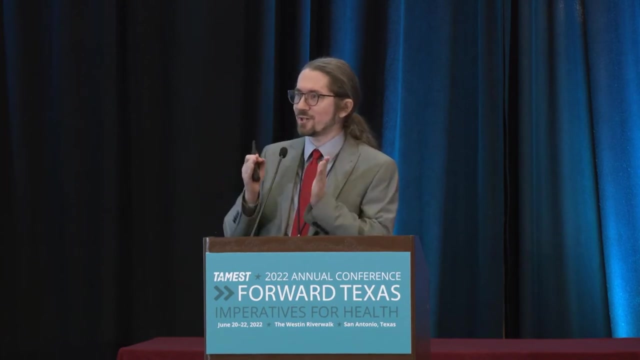 we inhale right now- and some of these pollutants can travel to alveoli and also to the bloodstream- The smaller the particle is, and I'm showing here, for example, the PM 2.5 and PM 10, how it relates to the diameter of human hair. 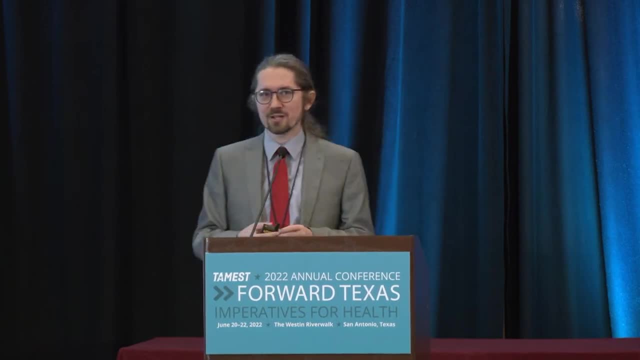 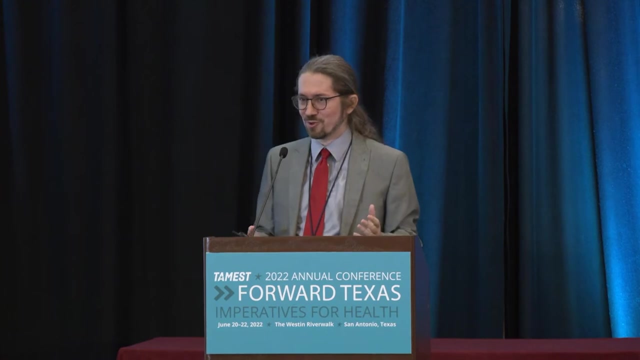 And the processes indoors are pretty complex. The indoor air environment is quite different than outer environment, And one thing that is different is that the volume of the atmosphere, of the outdoor atmosphere, is enormous compared to indoors. The volume of indoor spaces is so much smaller. so different pollutants can accumulate. and what's important is this Q, so ventilation rate. So this ventilation rate is basically an air exchange rate, so the rate how many times the air is exchanged in space, and the volume. so the volume matters too. 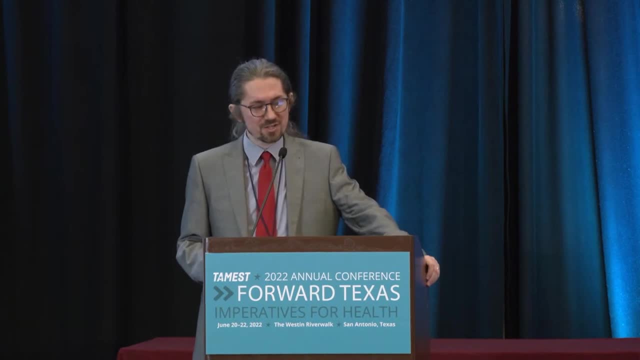 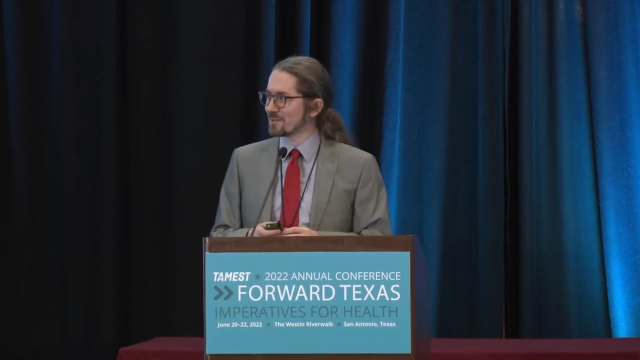 So what are major Major indoor air pollutants? And here I will show you some research from the UT test house. We are very lucky at UT Austin to have this wonderful resource And that UT test house is one of the most characterized houses on the planet. 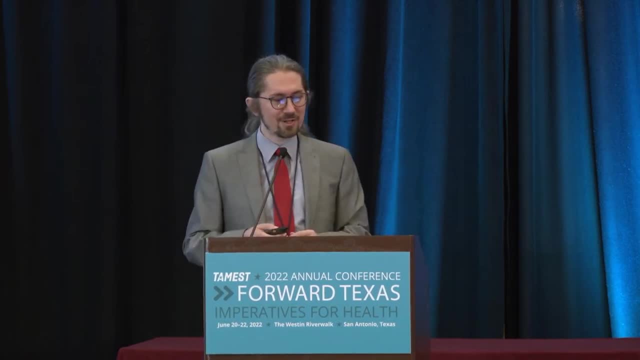 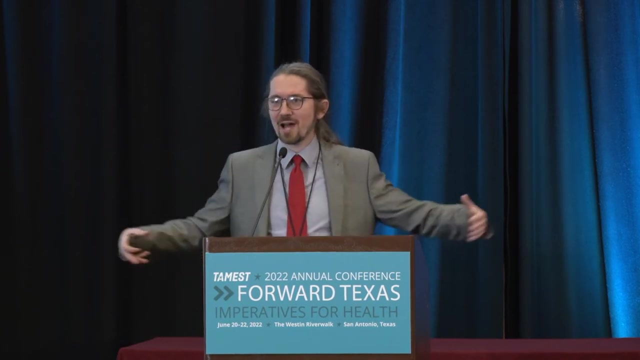 So you can do whatever you like in that house We had. we hosted a large campaign. Top researchers from all over the world came to Austin and what you can see here on this picture is basically. UT test house is surrounded by trailers with million dollar worth instrumentation. 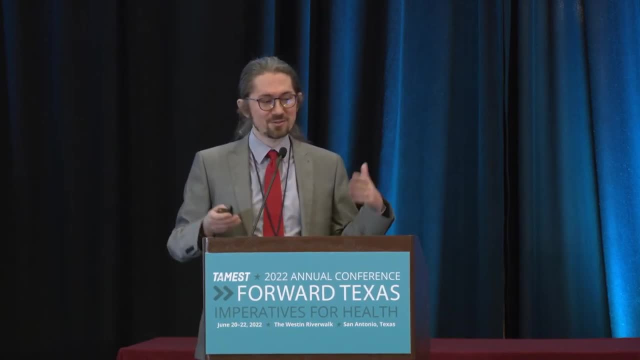 that's basically looking at what people are doing. So it's a conventional, normal house and we did something as cool as stir fry experiments. but also many, many papers you can read from this campaign, And I will start from particles, I don't have time to go through. 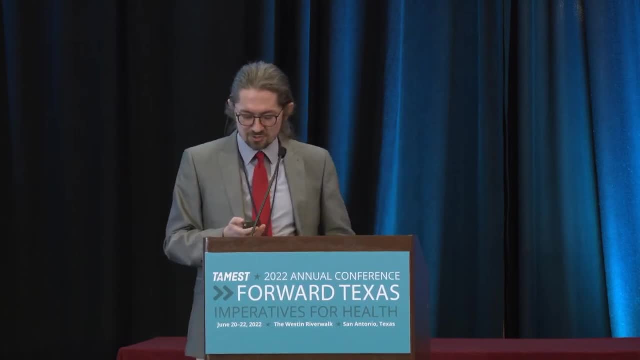 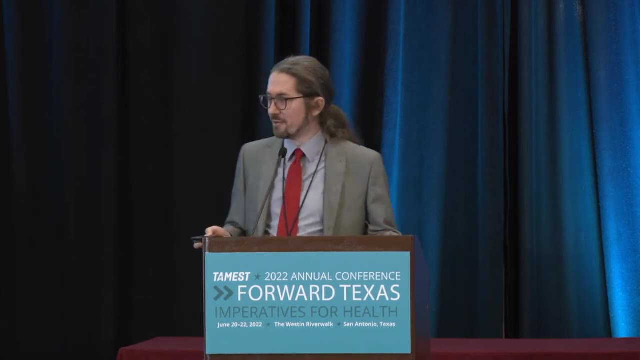 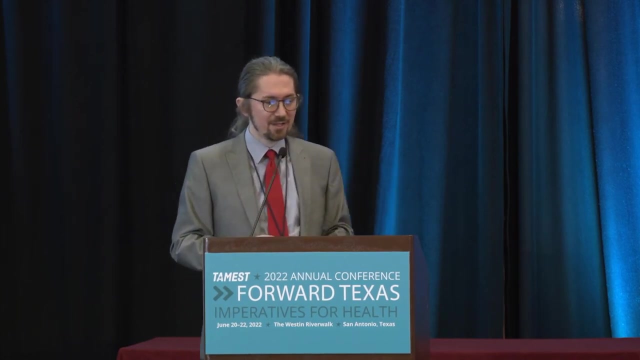 all the details in this graph, but what I want you to notice, that each time there was some cooking event, for example, or cleaning event like mopping, the number of particles pretty much went through the roof And it's the size as I was showing you. 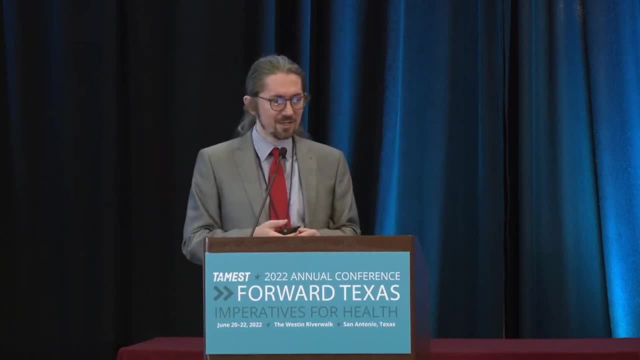 the alveoli is important And, as you can see, different foods will generate different size distributions And so, for example, if you look at the toast, it's shifted more to fine and most others are ultra fine. The composition of particles on the right. 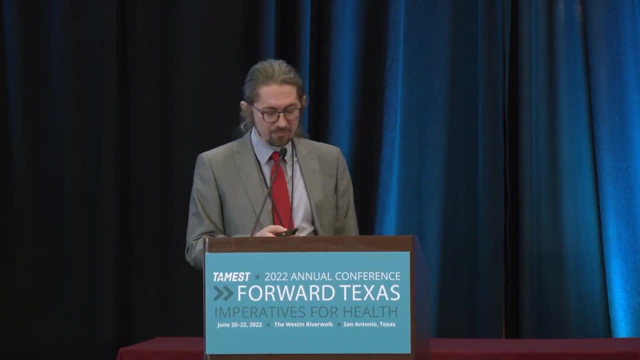 is also important for human health. So what about gases and gas phase pollutants? We know the famous Paracelsus quote is that the dose that makes the poison. And this is an important fact because we have, as I mentioned, we have thousands of pollutants. 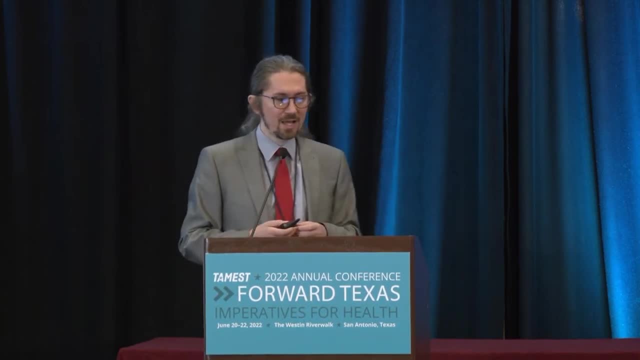 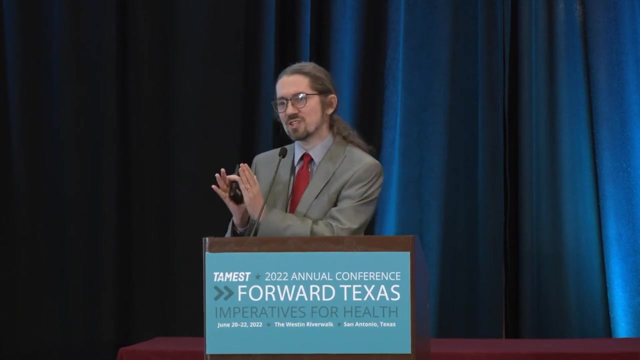 that we are inhaling right now as you listen to this talk, And the abundance spans nine orders of magnitude, but so does toxicity, atmospheric lifetime And our level of understanding is skewed towards most abundant compounds. But the most abundant compounds, I'd use them. 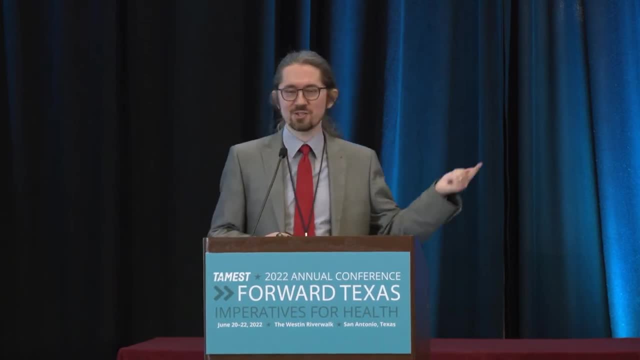 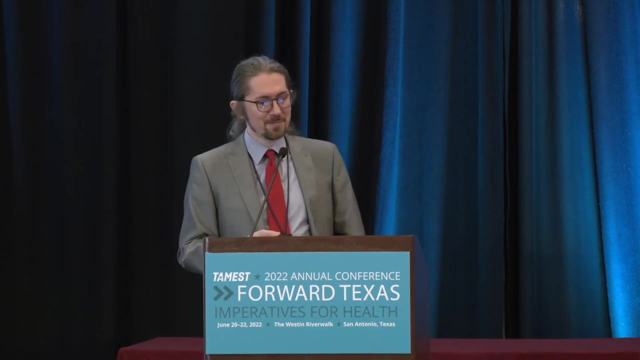 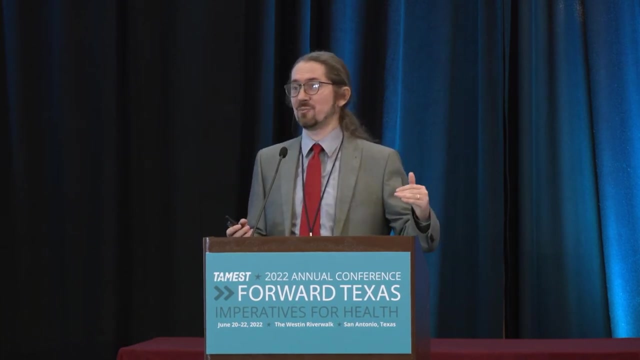 are usually not toxic, For example, ethanol, citric acid. these are compounds present in kombucha. I drink a lot of kombucha. I'm not really concerned about those compounds. I'm much more concerned about toxics which are below the detection limit. 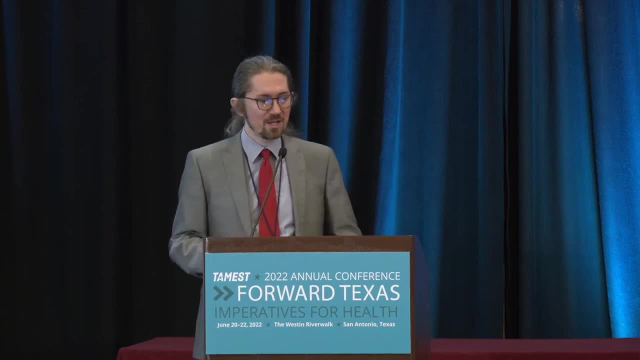 that we don't even realize that we get exposed to. So with better technologies that we have now, we are able to resolve even trace level of pollutants. The nice thing about gaseous air pollutants is that you can fingerprint pretty much every single activity. 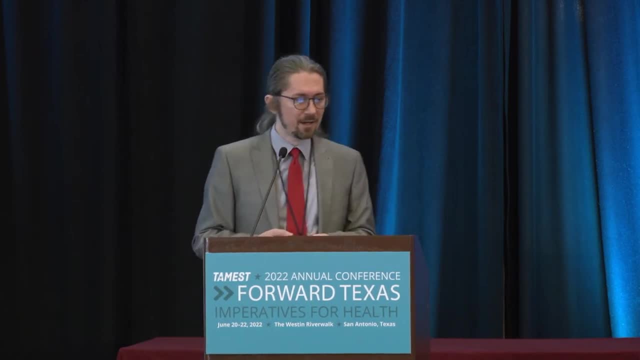 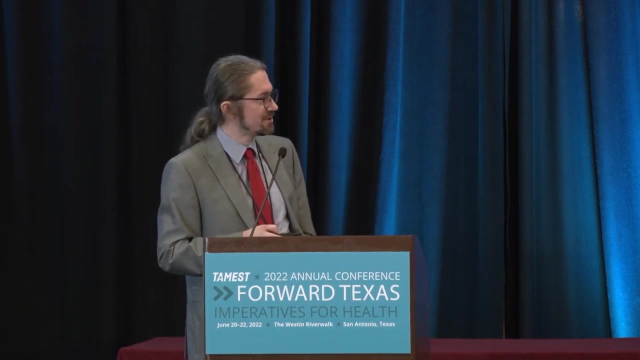 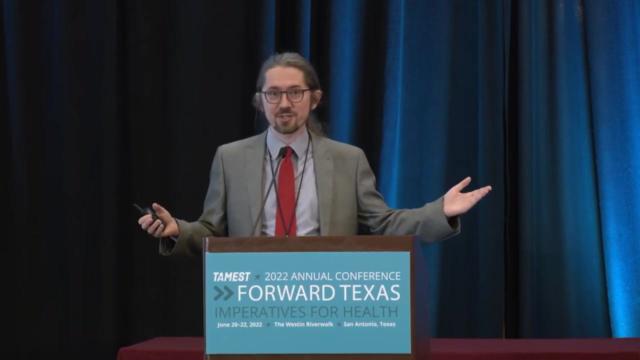 every single source. as you can see here, bleach, mopping and stir fry have different signatures. But what's blowing away is that the outdoor air quality, this gray portion of the pie chart, is really minor compared to all the other sources that are indoors. 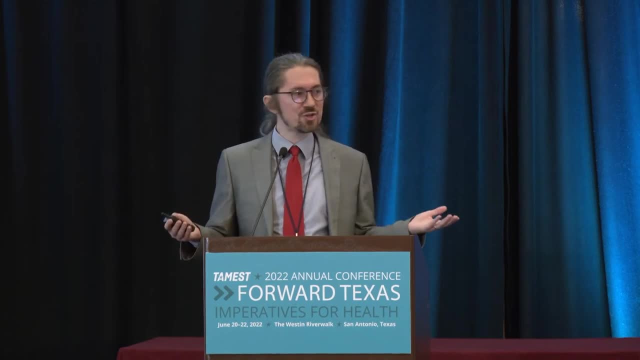 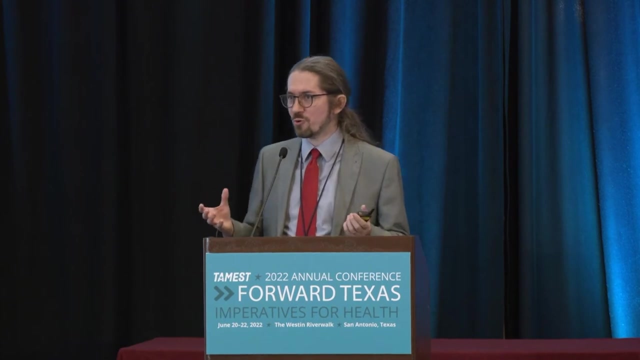 And historically we focused on characterizing emissions from building materials. But even building materials constitute less than a half of emissions, And it's cooking and humans actually dominate quite a lot. It's another half of the pie chart. So historically the approach was: 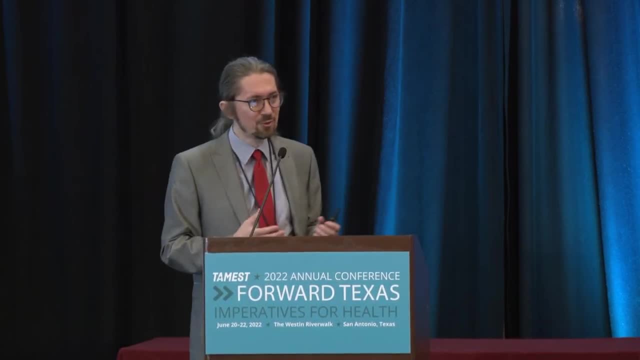 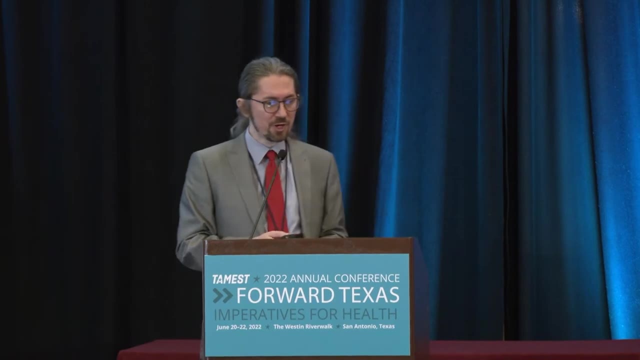 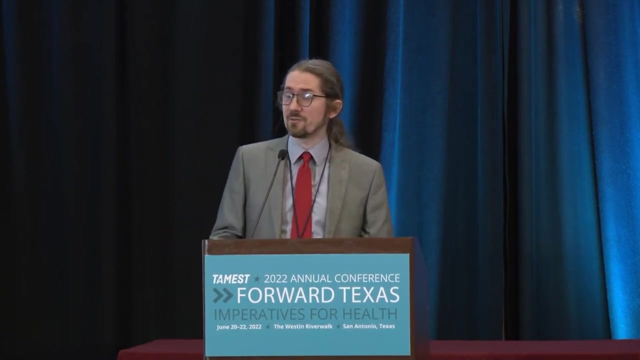 to go to as many houses you can and do a snapshot. Just take a snapshot. composition of indoor air And this is one of those very nice classic papers showing select number of different volatile organic compounds, including toxic benzene, exposure to which is very well known and characterized. It's. It's linked to leukemia and cancer, And what you can see on this graph is that quite a large portion of houses have very high level of benzene, And you might be thinking, oh, maybe those houses use a lot of benzene or products like paint. 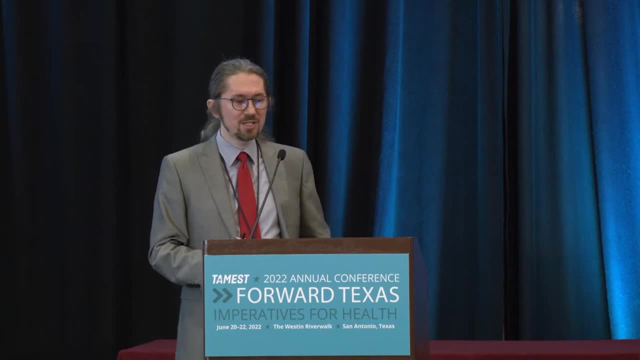 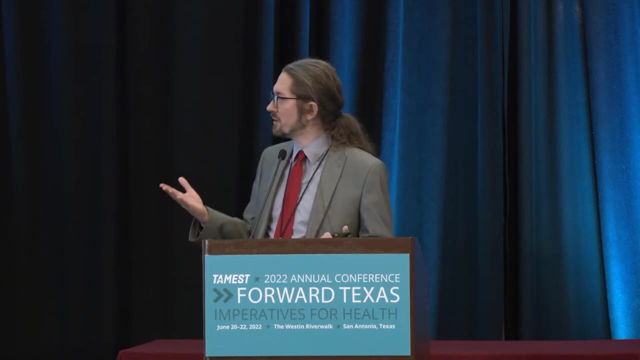 and so on, which is probably true as well. But what this graph actually is reflecting is how well the spaces are vented. So the well-ventilated homes will have much lower benzene. But we can do a different approach, So the novel approach is to find just a few houses. 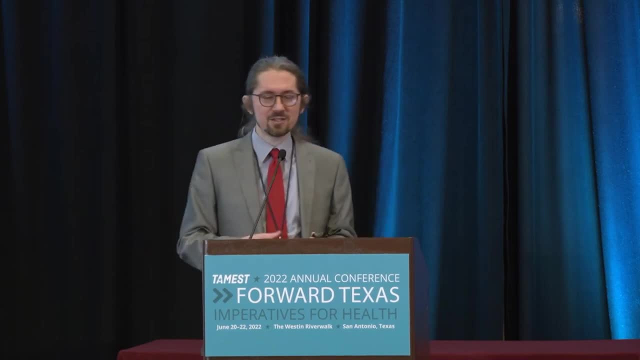 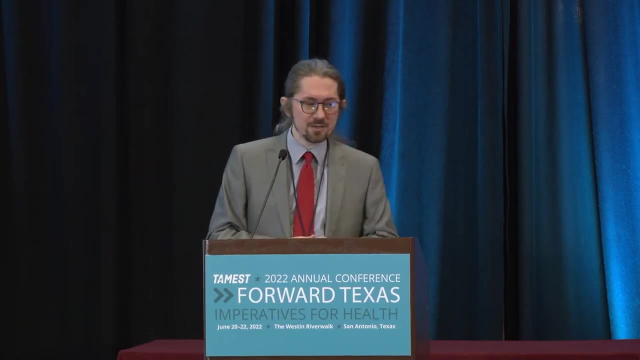 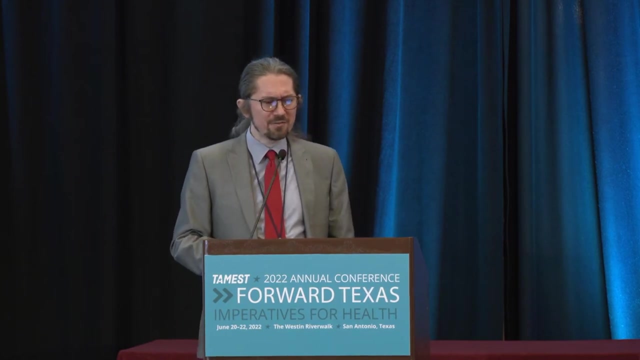 which are representative and continuously measure what is happening in different spaces, And here what we did in Oakland Hills, for example. It's a very nice house. We even wondered if you will see it. look for some clues. It's a well-ventilated building. 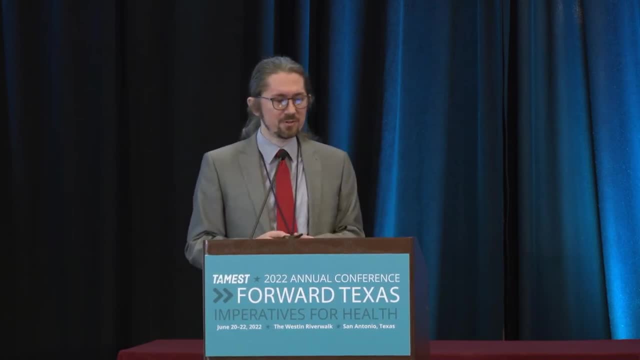 will see anything there And for a period of more than a month. we're continuously looking at those different spaces. So if you look at the average mass spectrum- so this is campaign average more than a month- you can see that it's quite complex: more than 200 different. 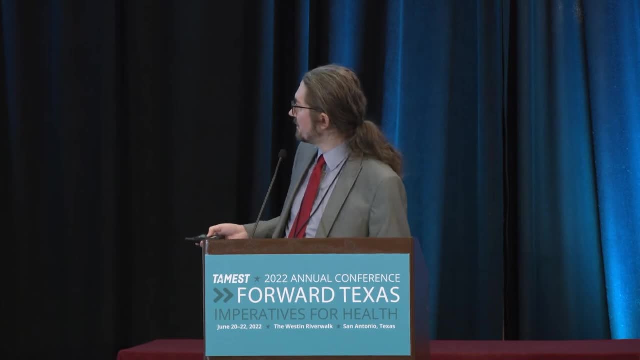 chemicals and you can see things like, say, loxanes from consumer curve products, different benzoins, furanoids and lots of different compounds. So what we can do, we can sum up these compounds and show us the total VOCs. So this is the sum of VOCs on the y-axis. 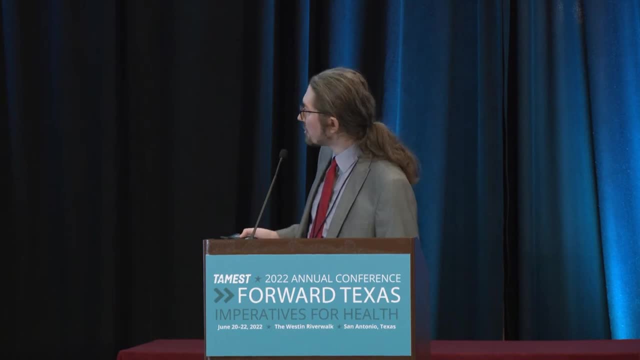 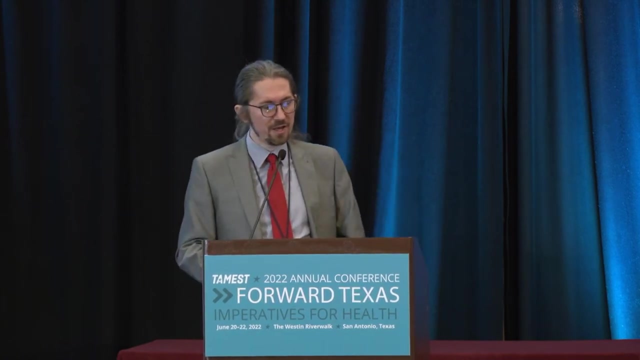 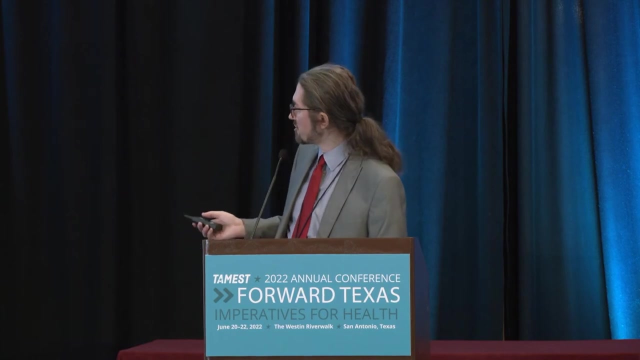 and this is about one month- and it's colored, And this is colored by carbon dioxide, So carbon dioxide originates mostly from breath In the outer atmosphere. it's about 400 ppm, And what you can see here is, whenever people are present, the concentration is super high. But do you know what's in here this lowest? 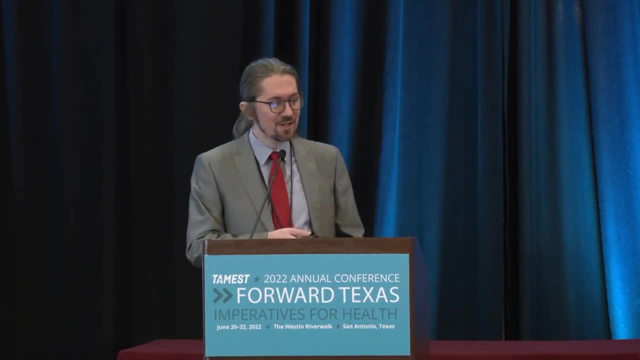 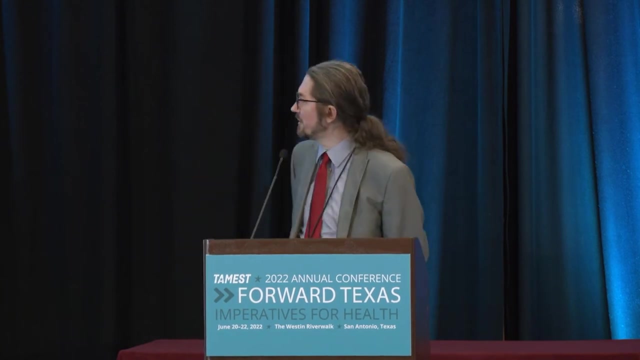 point on the graph. Well, this is. This is actually when occupants opened all the windows and all the doors. This was so called a ventilation experiment. So this is only when you can really reduce the concentrations to levels close to outdoors. And do you know what that period is? This is when the house 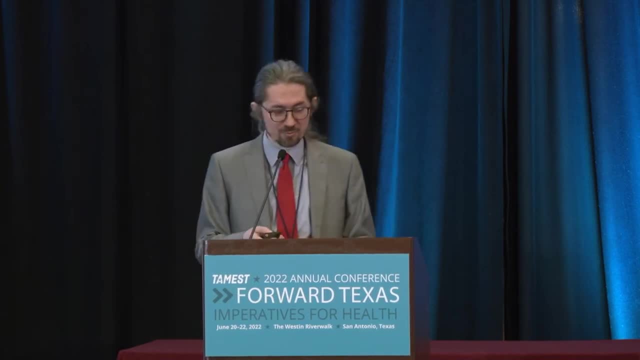 was vacant, The occupants went for vacation And so So to present it on the deal pattern like basically averaging the whole period of campaign, you can see that the outdoor air compared to indoor air, there's a huge difference. And if you look at other spaces- kitchen, hallway- it follows because there is good 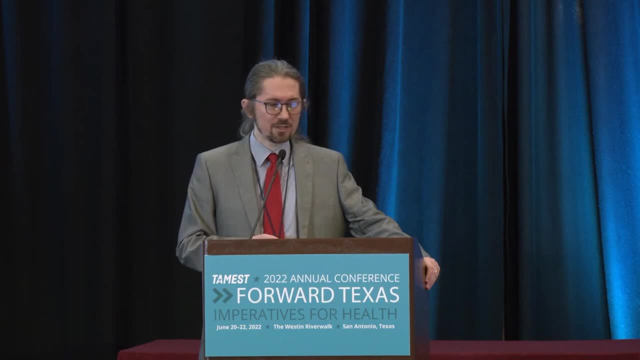 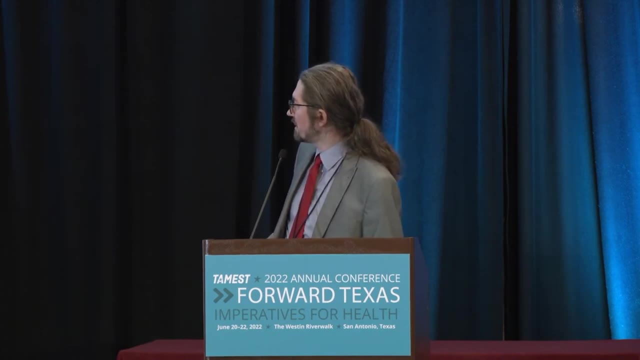 mixing. So another way to look at it is to look at outdoor and indoor air. And the reason why it's important to look at outdoor air is because you can see that the outdoor air is like zero air when the house was occupied and vacant, So outdoors it doesn't make a difference. 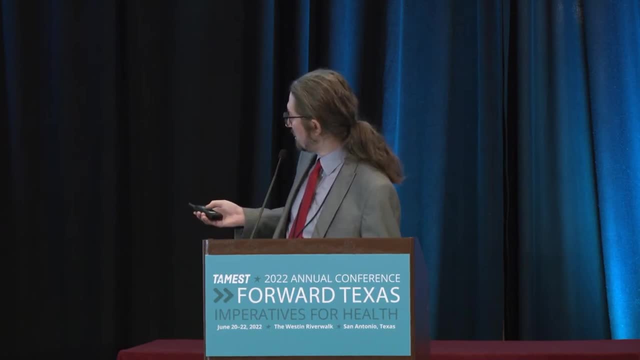 if people were present in the house. But as you can see indoors it's such a huge difference when the house is vacant And the standard deviation from that average is absolutely huge. As you notice, it's a different scale. Do you want to see it on the same scale There? 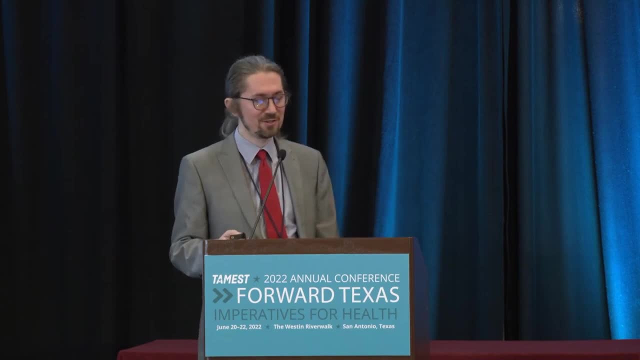 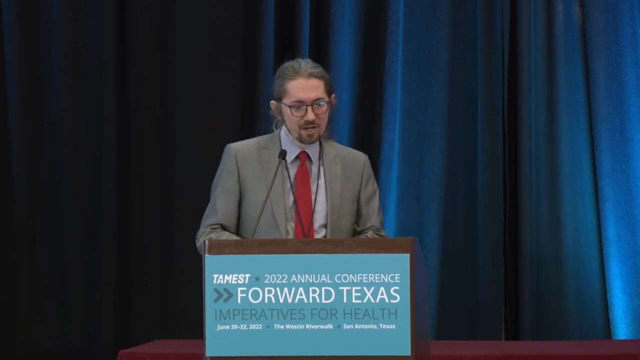 you go, The outdoor air is like zero air, literally. And therefore I come to the question: We know now that the air, indoor air, is generally more polluted than outdoor air, but how to embrace complexity of human exposure, to understand their effect on human health? And in my lab we are discovery-oriented and we really develop. 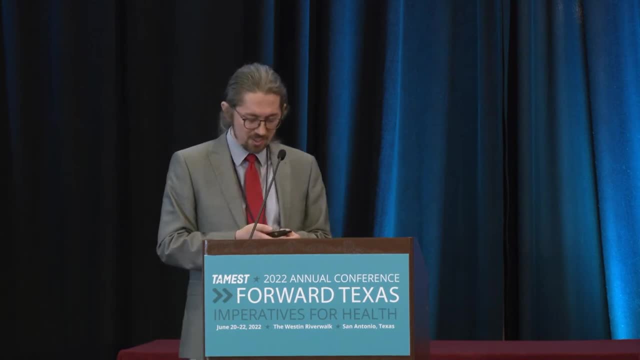 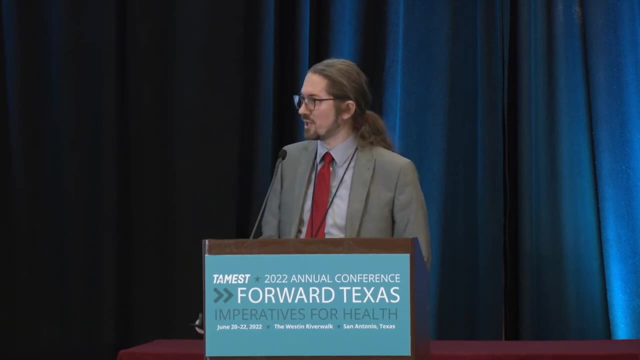 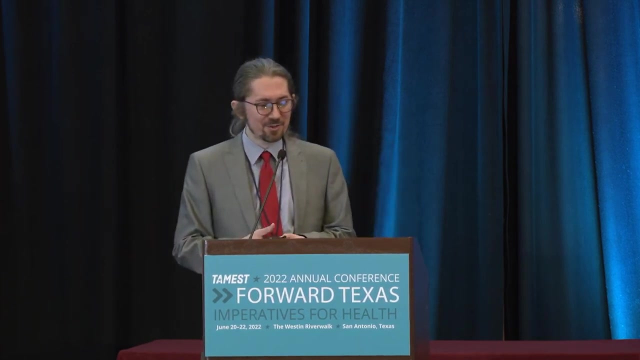 novel methods to look at air pollution. We have the very unique mass spectrometer called VOCUS-2, our proton transfer reaction time-of-flight mass spectrometer, And this is a long name, so we prefer calling it the sniffer, And the sniffer is really cool and it's a similar. 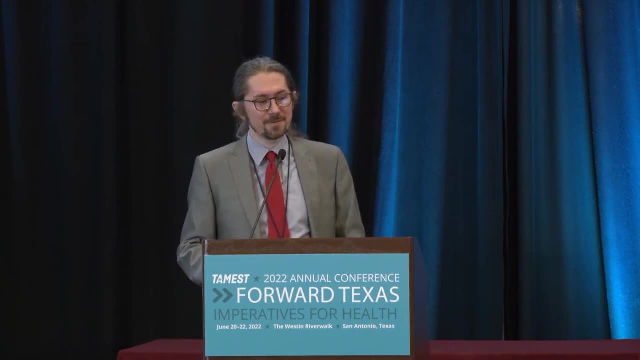 instrument that we used in Oakland Hills that I showed you the data, but it's like the newest generation, It's like a Ferrari among the mass spectrometers. There are only a few of those in the nation, So I'm going to show you the data. 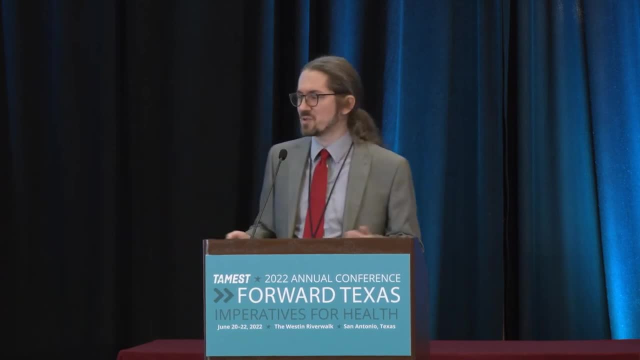 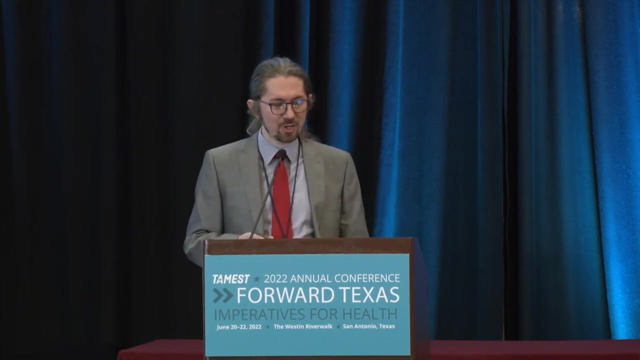 Just as an example, schools have spent a lot of time and a lot of effort and funding trying to make spaces clean, and that's definitely a good thing. But the question is: should we care about what's in our cleaners? Are there any risks of disinfectant exposure? So just when COVID hit, we had this idea. 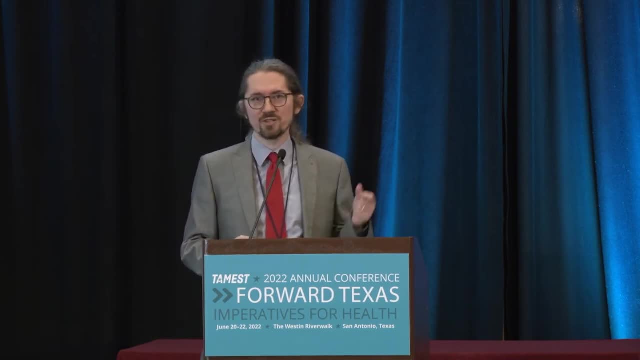 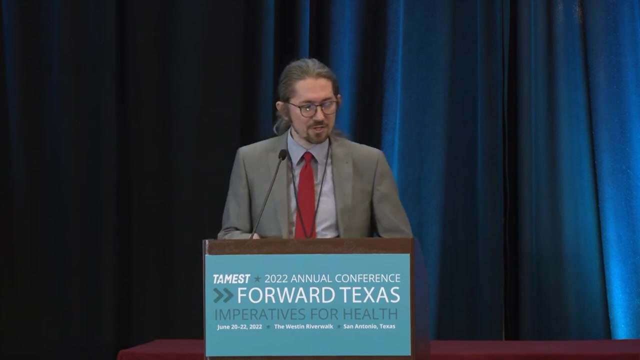 that we wanted to know what is happening when we disinfect spaces, what are the byproducts and what is the role of masks. So we conducted quickly a pilot study and got funded. The PIs are Leah Hilderbrand-Ruiz. 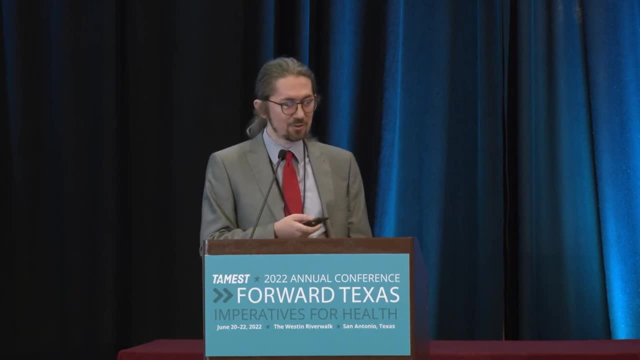 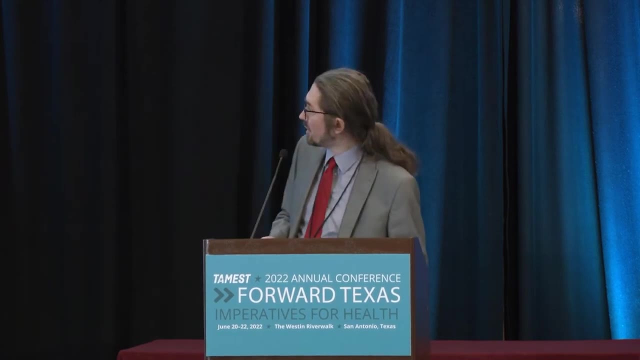 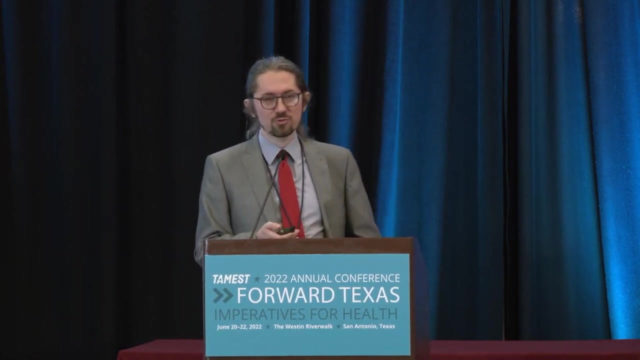 Attila Novoselak and myself, and also a lot of students, had a lot of fun to work on this research. So I will just highlight some work of my outstanding PhD student, Daniel Blumdahl. So basically, to understand exposure, to quantify exposure. 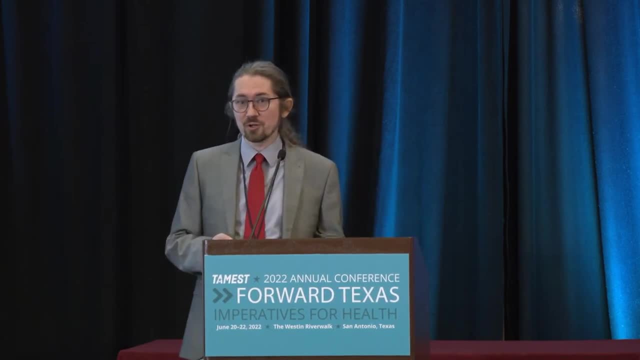 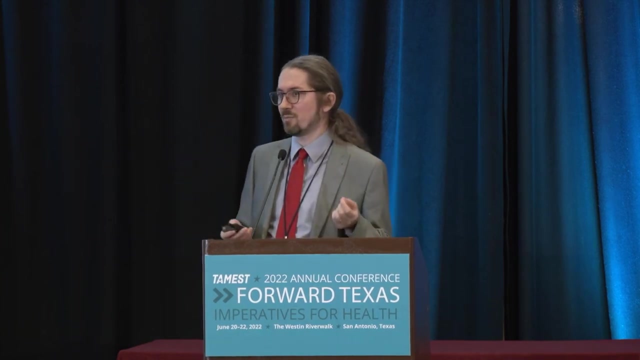 what you need is to measure concentration, but also what you need is time. So this area under the curve. if you, for example, want exposure for one hour, this area under the curve is equal to exposure And if we use the dynamic mass balance model, 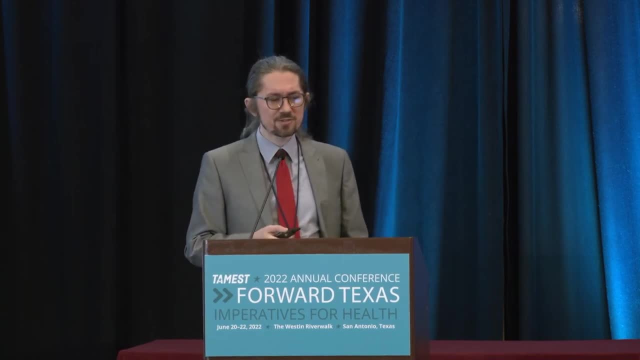 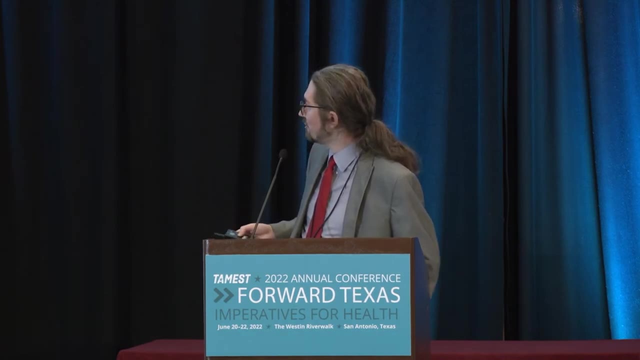 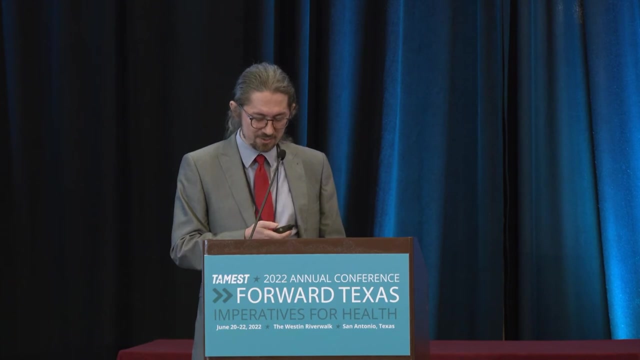 on the indoor space, you can see what a huge difference it makes to this area under the curve if you have a tight envelope. So this is basically when you don't ventilate the space very well and when you have more ventilated spaces. 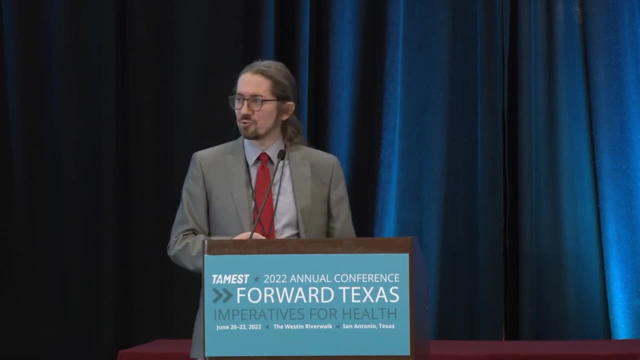 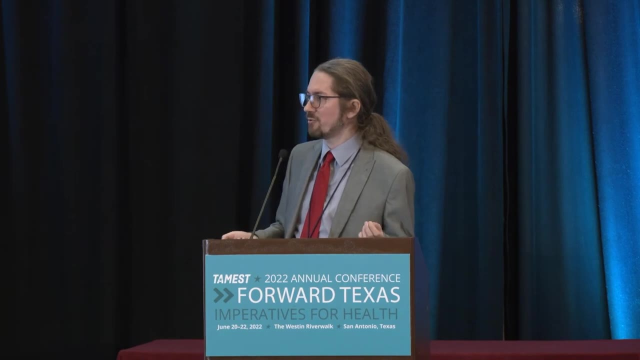 So definitely a huge effect of ventilation on reducing exposure. So what about the masks? Do they make things better or do they make things worse? Well, of course, for disinfectants, And here is on the upper graph shows dichloramine. 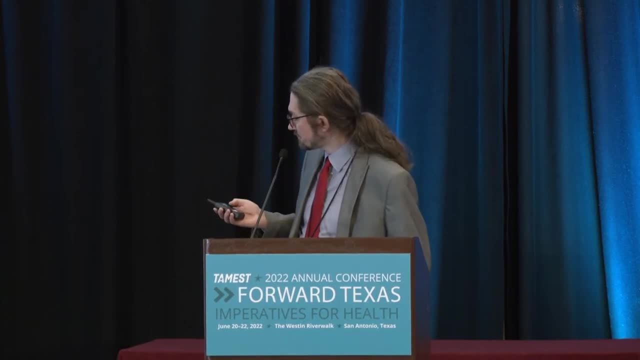 It's one of the byproducts formed in bleach disinfections, And the open squares correspond to a concentration in front of the mask and the closed circles correspond behind the mask. So you can see a huge reduction in exposure for dichloramine, which is relatively sticky. 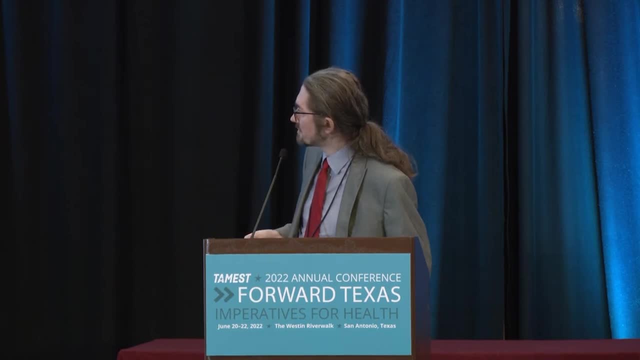 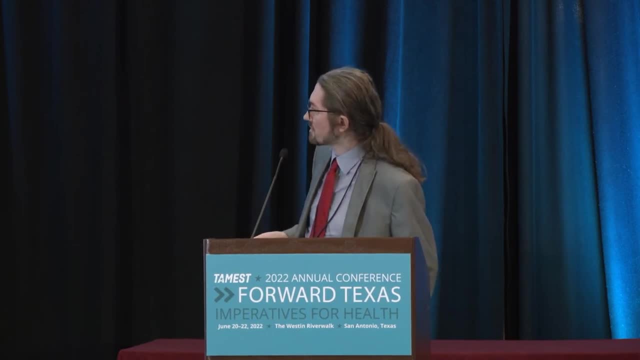 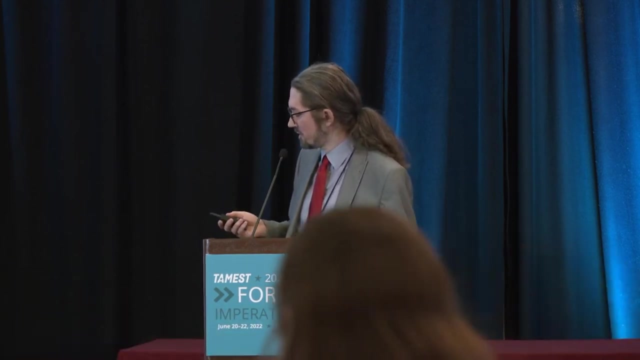 But after some times there is accumulation on the mask. So what is happening? if you don't get rid of the mask, the exposure actually from using the mask will be higher. So if you use the mask, you need to remember to to dispose of it after the cleaning event. 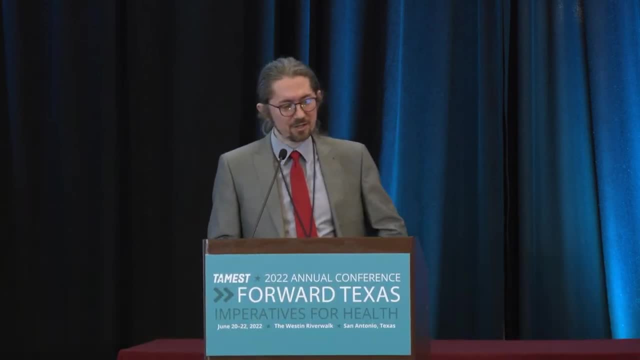 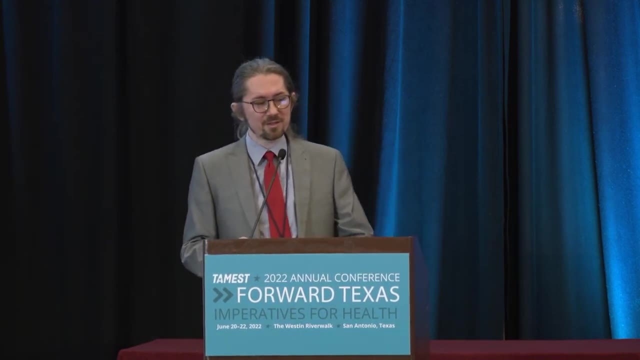 So one discovery my other student made on other projects, when we looked at microbial VOCs in indoor air, something that she discovered was that when we change relative humidity- so this is about learning about the fundamental process indoors- When we change relative humidity, which is generally the case- 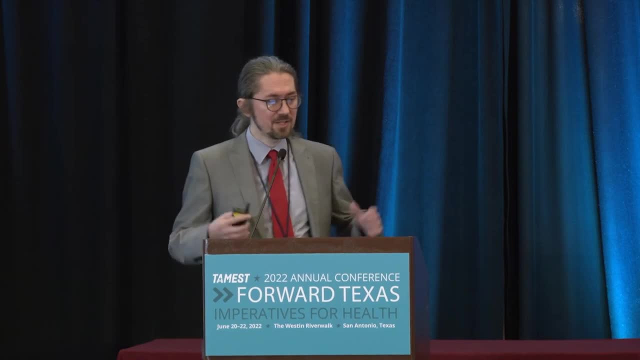 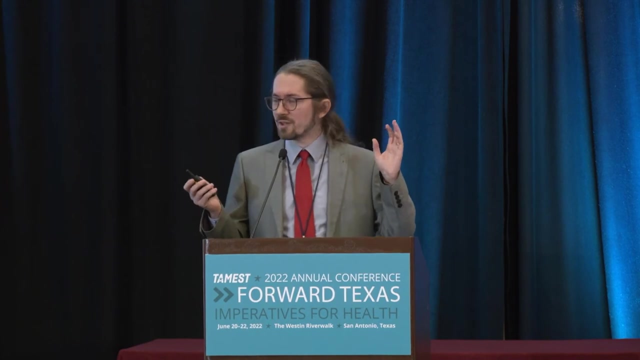 what it does is that this drying and wetting process. it results in higher emission of material degradation markers, So we can actually track degradation based on the specific markers, such as morpholine type of compounds coming from polymer like nylon, for example. So okay, so would the best approach be to actually measure pretty much everything? 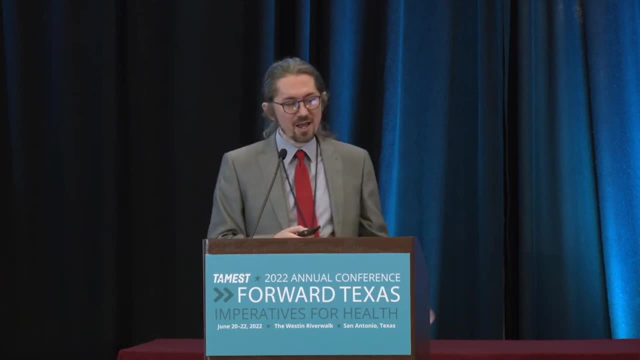 in different air spaces and do we measure everything? And the question is that it's not sufficient. I think We also need to monitor Some metabolites. so basically, we could monitor blood for some air toxics that we got exposed to, but there could be some other novel methods. 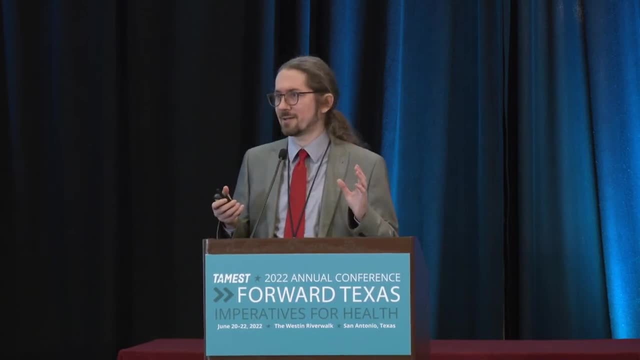 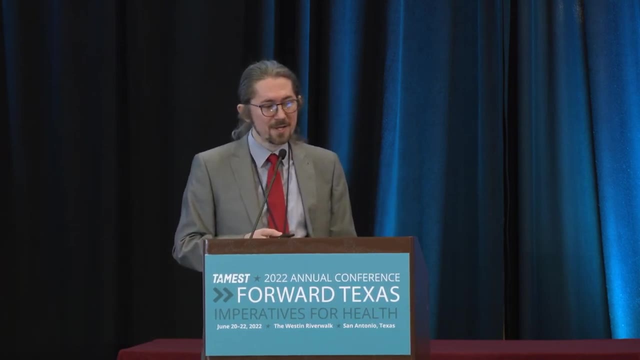 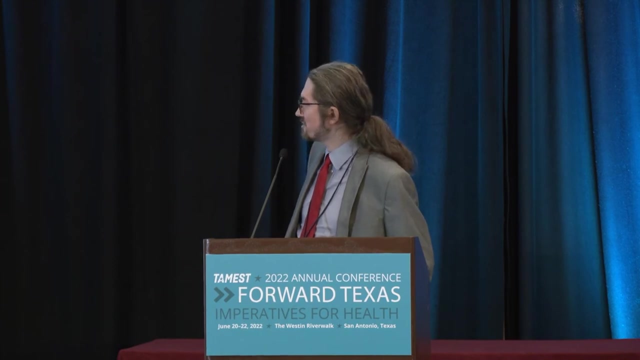 For example, in my lab we have a breath inlet and we can look actually at breath metabolites. So human breath analysis seems super promising. and this is a quite complex graph but I want to walk you through carefully because it's really, really cool. 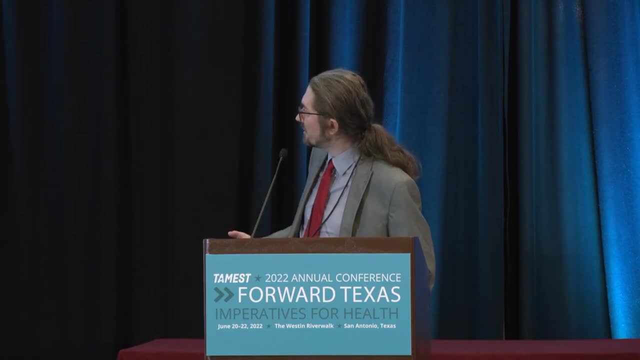 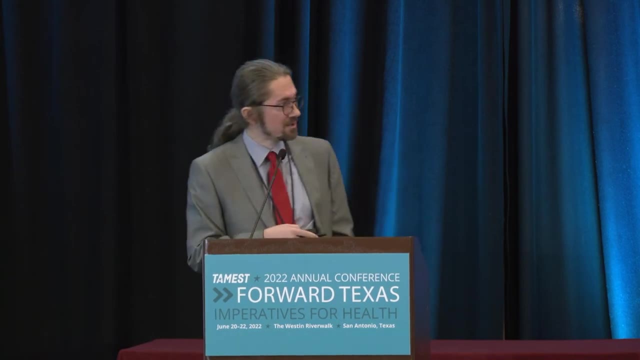 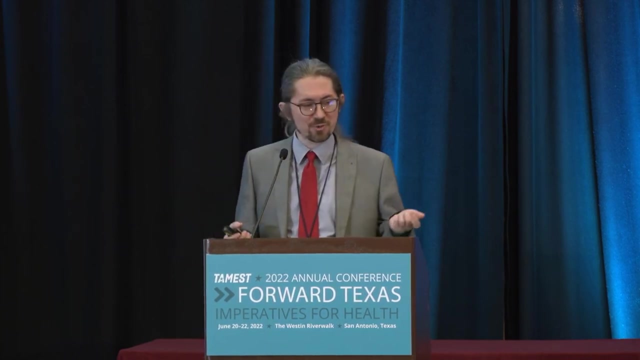 So this is a log concentration ratio of exhaled air to inhaled air. So what you see on the upper portion of this graph is what is enhanced in breath. So, as we expect, we see metabolites such as isoprene coming from lipid metabolism. 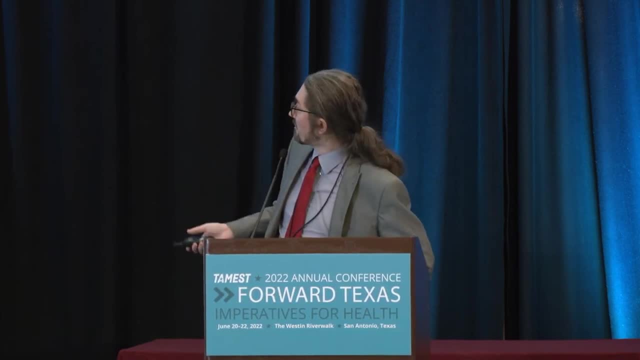 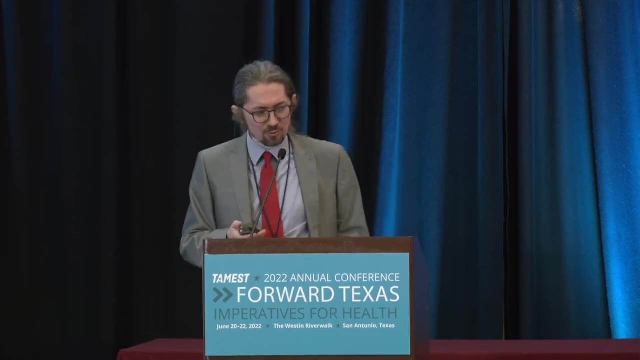 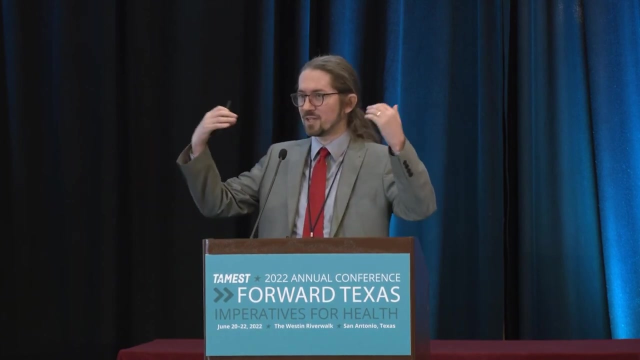 sorry, sugar metabolism, acetone coming from lipid metabolism and so on, And also lots of other metabolites. But another cool thing is that we don't just exhale endogenous metabolites. We exhale pollutants that we get from the environment. 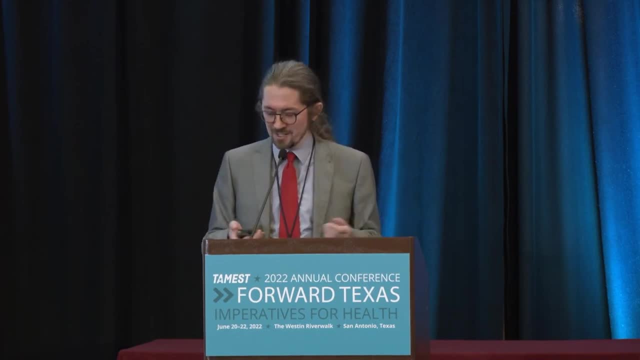 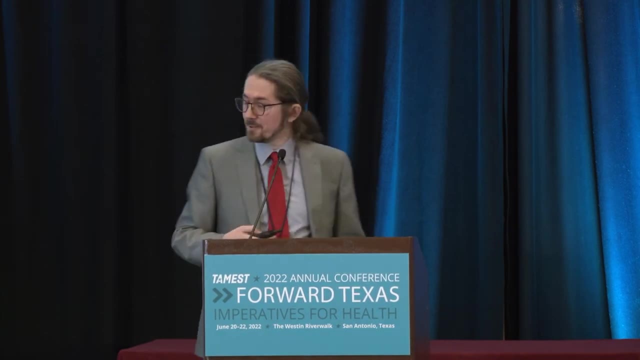 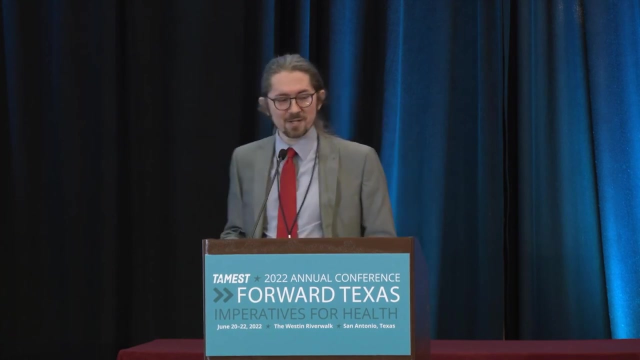 And because our inhaled air is not clean air, we also exhale air toxics actually, such as aromatics, And for example, here is D5, decomethylcyclopentasiloxane. These are compounds present in consumer care products. 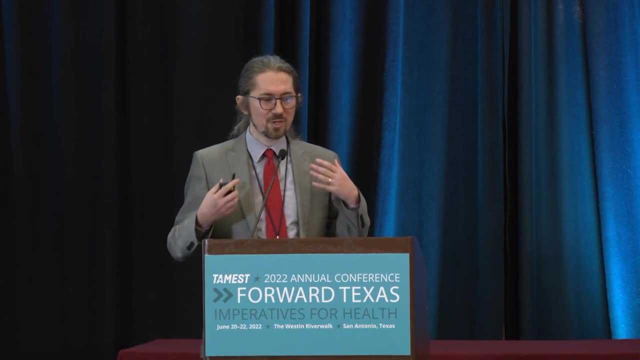 Source control is definitely important, But because we cannot stop exhaling, cannot stop certain emissions, we need to have good ventilation systems And at UT Austin we have the amazing full-scale HVAC system where we can study chemical processes, ozone-generated, the different byproducts. 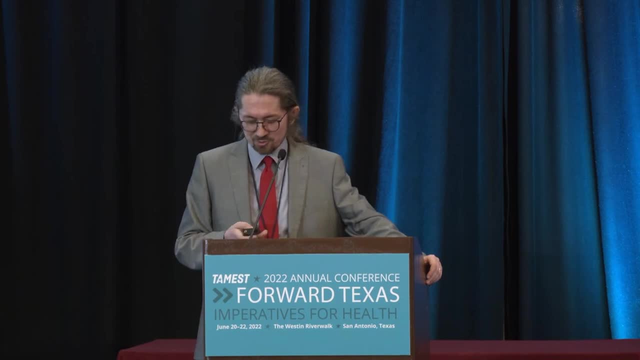 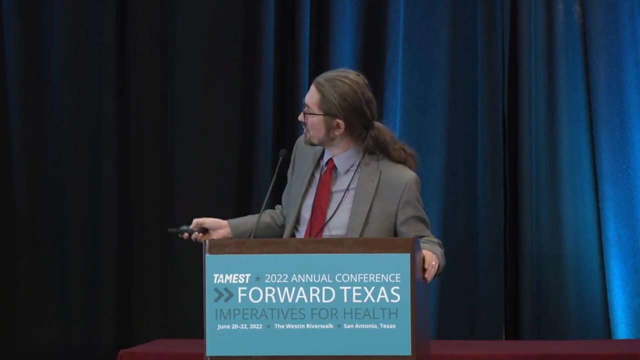 and also how efficient the filters are. I won't go through All the details, but this is just an example of an extremely efficient filter. You should. if the filter is efficient and it's compound-specific, you should see everything on the left. 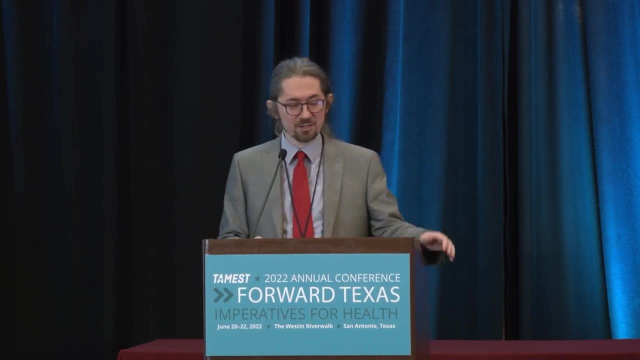 And this is the filter that is used in surgical theaters, in clean rooms and so on. So, anyway, just to summarize: the fact that the indoor air quality is unregulated it doesn't mean that it has no effect on human health. 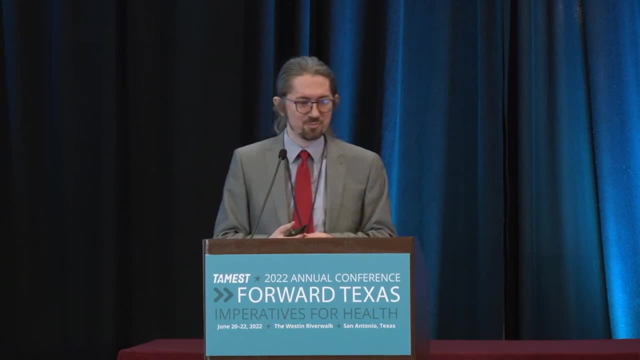 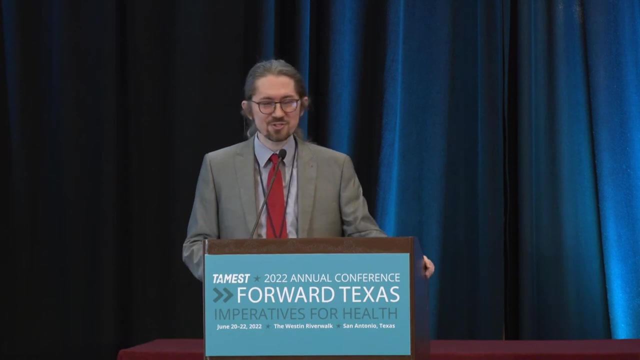 We need more studies, We need novel measurements- Both of Okay- And we need to quantify the link between exposure and human health. And in my lab we are pretty much obsessed with fingerprinting all the different sources. You know the saying: you don't walk to the same river twice. 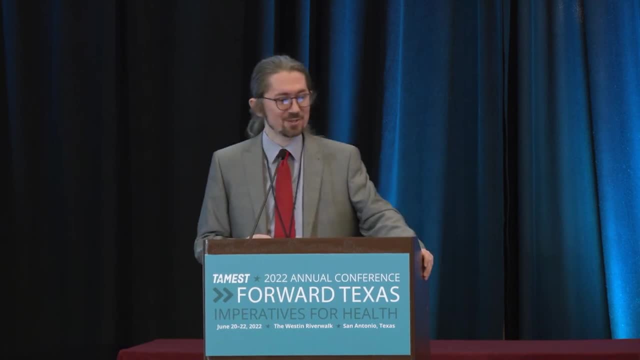 And I'm saying you don't inhale the same air twice. So with that we also have specific sources of exposure, like communities living close to oil and gas, And we also work to understand exposure of firefighters when the house is on fire. 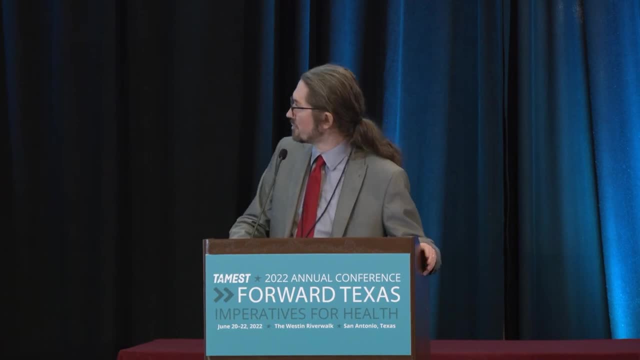 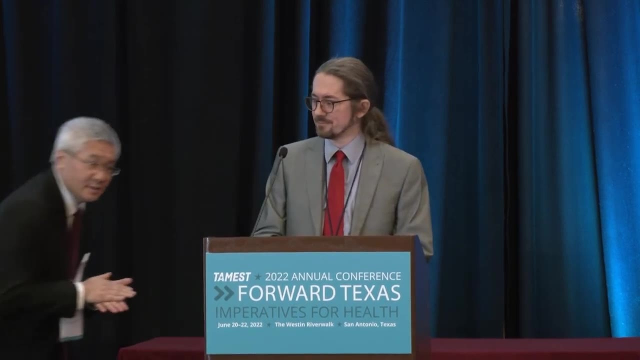 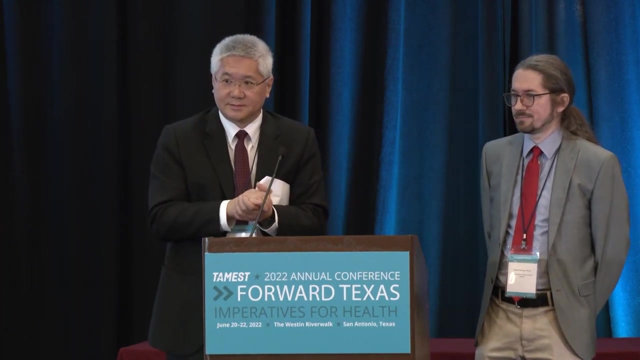 So with that, I would like to again thank all my research group and sponsors, And thank you all for your attention. Thank you, Dr Mistal, for that interesting talk. We have time for maybe one or two questions. Please identify yourself. 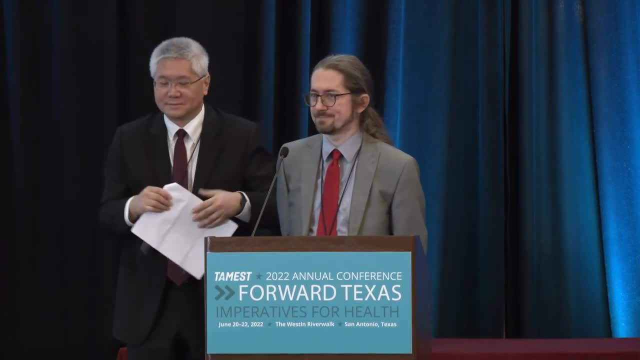 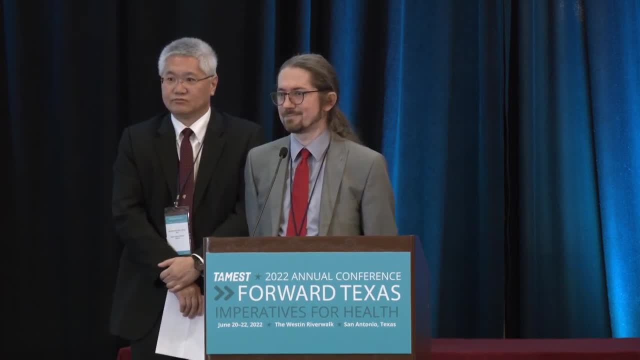 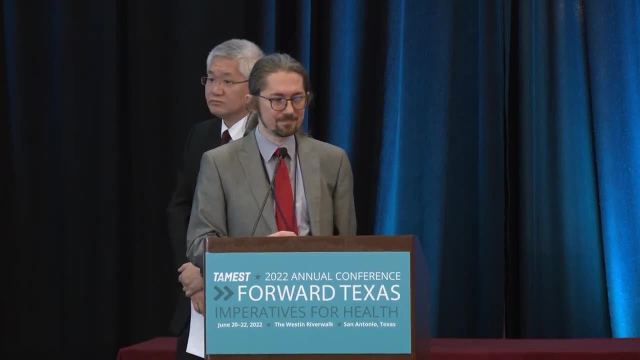 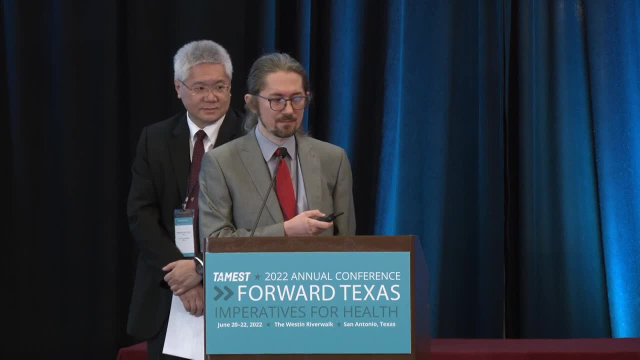 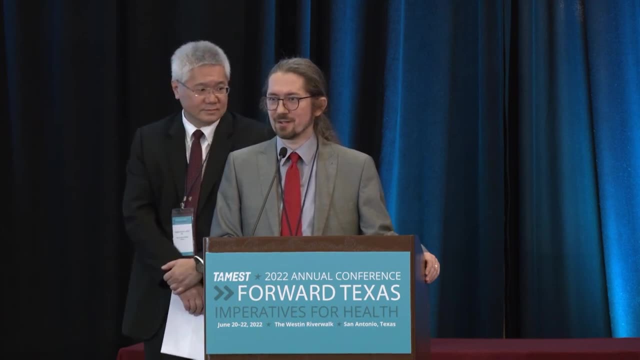 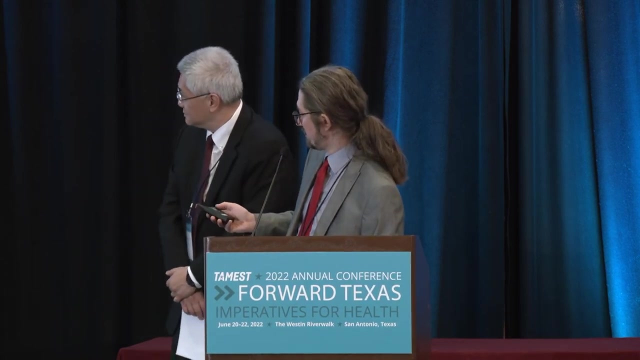 I think it said percentiles and micrograms per. yeah, this one, I was kind of confused. If you could explain this graph a little bit better so I have a better understanding, Okay, yeah, yeah, so this is like percentile of homes. so, for example, here you would have. 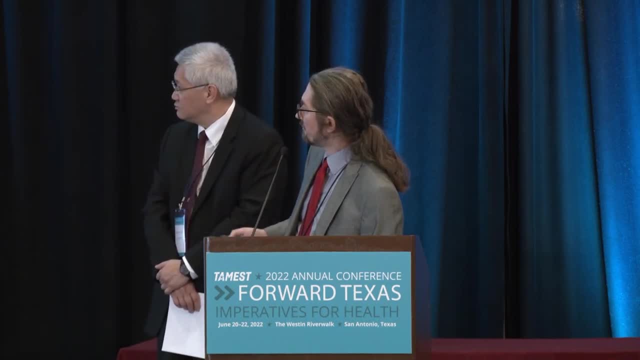 the median right, So the top. so if you had like two thousands of different homes- so you have a few hundreds which would have so somewhere, here is the recommended level for benzene exposure. So a lot of those houses would have exceeded those benzene levels. 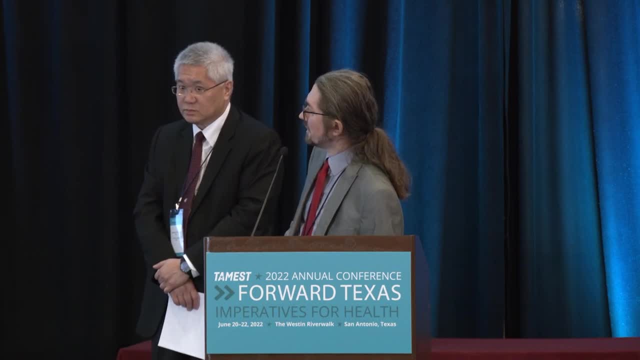 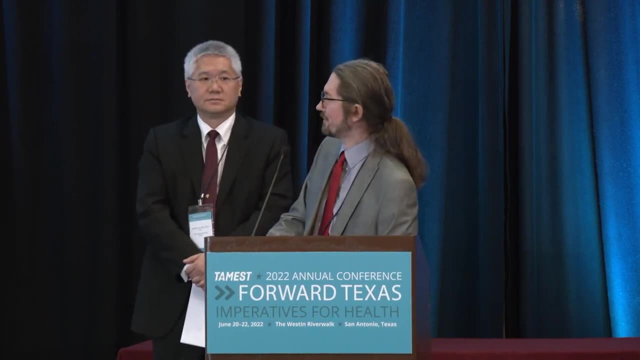 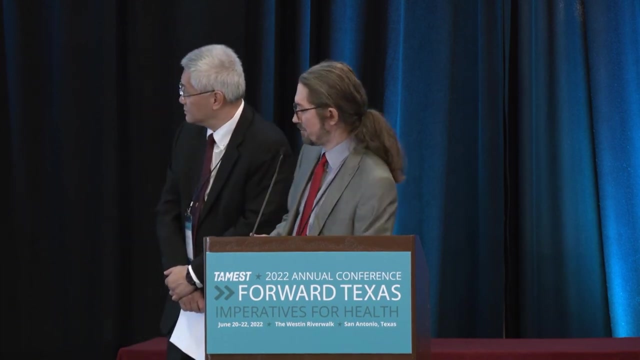 But because these were snapshot measurements, it could be that they were taken at different times of day, when people were preparing dinner or and so on. So in other words, 100 percentile homes have 16 micrograms per meter cubed. So this is like basically the level of exposure in different homes. 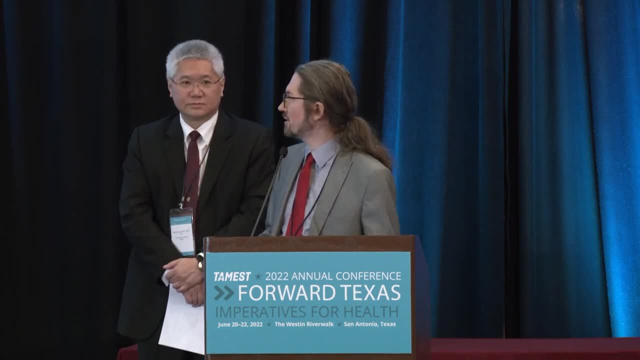 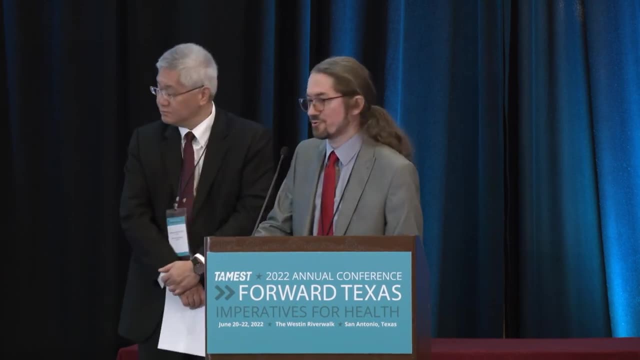 Yeah, So this is like the survey of select VOCs from like 200 and this is by. you can read up the paper by Zhou. yeah, Thank you. Thanks, Yeah, sorry that it was unclear. Hi, I'm Steve Ginerich. 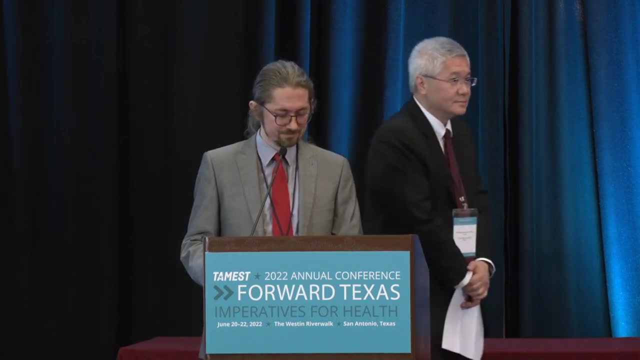 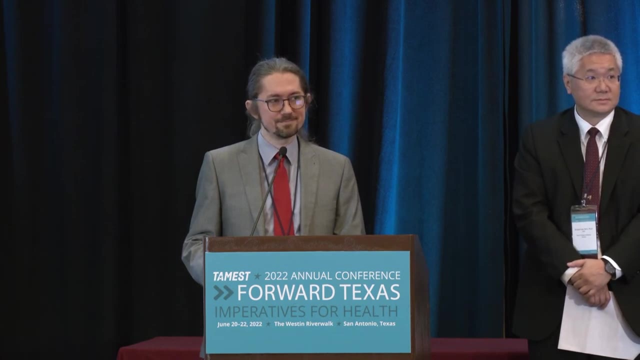 I'm with UT Dallas in our innovation and commercialization area, And we're about to open, with the city of Richardson, a new 30,000 square foot space that has as part of it An installation of technology by a company called ActivePure, with filters throughout. 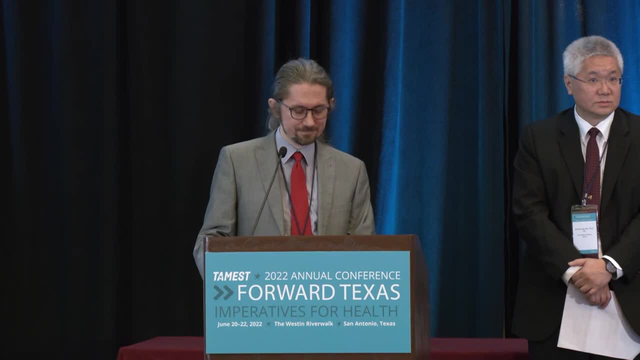 that has a degree of FDA approval for some of their filtration technology. But what I'm interested in is the efforts that you and other colleagues, either here in Texas or elsewhere, are pursuing to get lower cost versions of your sniffer technology, Because we have low cost versions of sensors for external air quality monitoring. 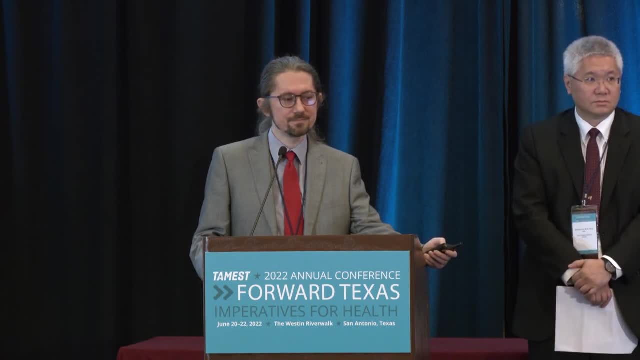 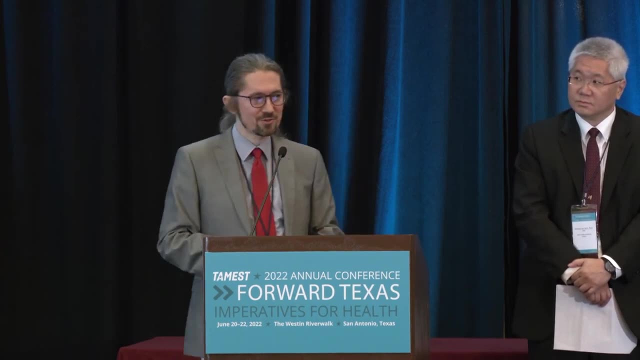 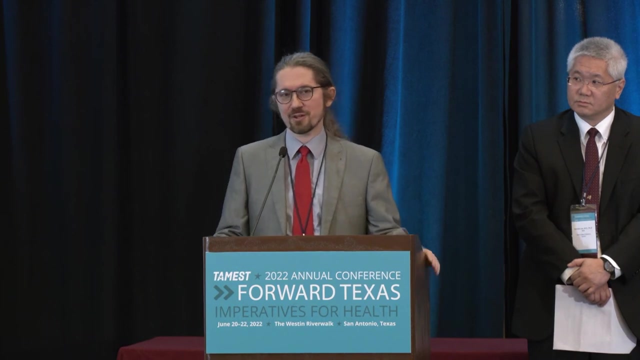 But I'd really love to see something low cost with high fidelity for the sniffer. So would love to hear your thoughts on what you're doing and what others are doing in that area, Thank you. Thank you so much for this question. So definitely the idea is to also have local sensors.